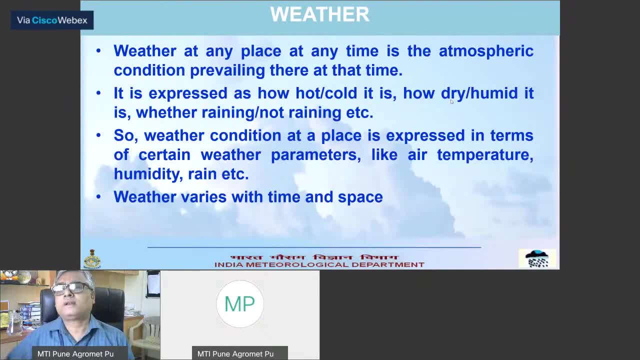 Thank you for watching. Thank you for watching. I will start with the very difference Weather. we all know It is the atmospheric condition prevailing at a place at a particular time. That is the weather at that place at that particular time And we all know generally weather. 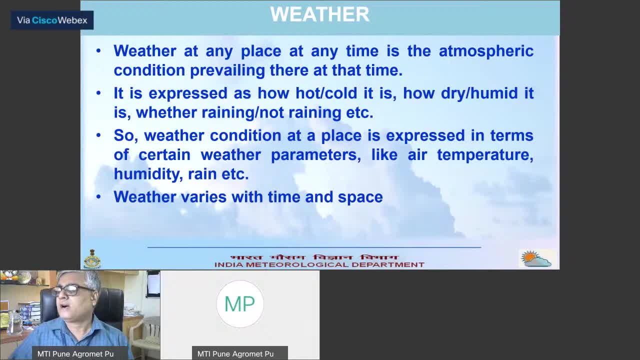 at any place, at any time, which is expressed as how cold it is, how hot it is, how dry it is, how humid weight it is, whether it is raining or not. so therefore, uh, therefore, from this expression itself, it is clear that weather at any place, at any time is expressed in terms of the values of 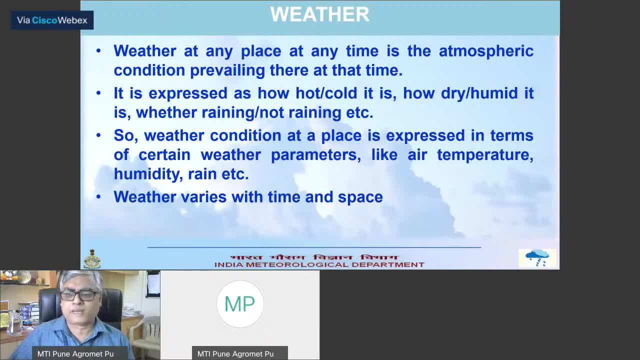 some meteorological parameters- we say weather parameters- like temperature, winds, speed or direction, humidity, etc. and we all know weather varies with time and space. because of the fact that weather parameters varies time and space mathematically, i request you to please mute your microphone. yes, sir, disturbance. 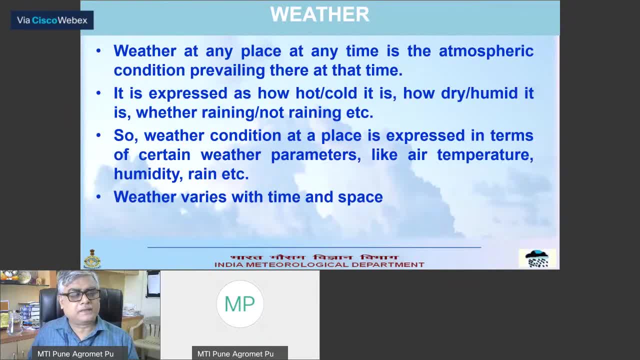 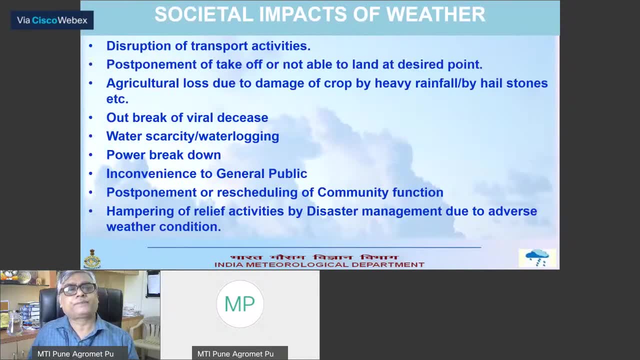 mathematically, we express it by saying that weather is a function of longitude, latitude, altitude and time. weather has significant societal impacts. a few of them only have been listed in this transparency: transport activities disruption, postponement of takeoff or landing, or we are trapped you. agricultural loss due to heavy rainfall or hailstones. 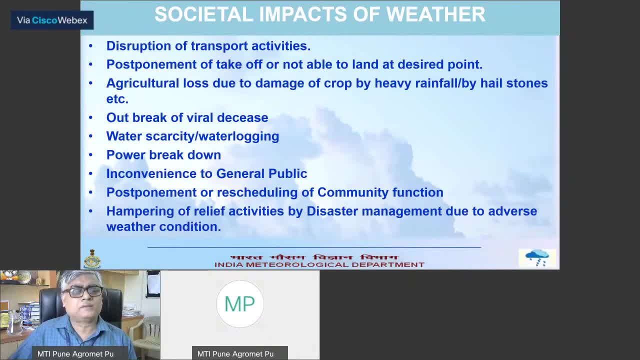 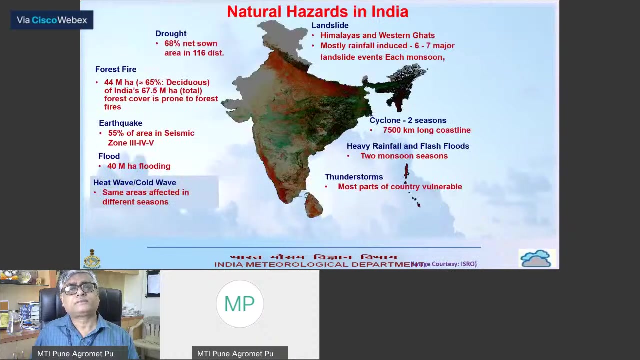 then viral disease, outbreak, water scarcity, water logging, power breakdown, postponement or scheduling of community function, hampering of the relief activities by the authorities due to adverse weather condition, which which were, which were, which happened during arm fun period, very much well known, upcoming more, if any. well, well, this one is: this is actually. this is a natural hazard. the natural hazard, say, in different natural residents: drought, forest fire, earthquake, flood, heat wave, thunderstorm, heavy rainfall, cyclone, lands, last, you'll see, except this forest, except this assignment that will stop a medium shock, transport atau storm, a big main for a cycle of landslide. youl see, except this forest, except this earthquake, all other are the only advantage that more and more number will be available. we must always consider, as he said, things will expand in the near future, so as the information more and more 하는데 take into account, if you, we do not, we must work for this time in the nearest possible and develop, build a flood, an abundant garbage, vitality and lot. all this, we do have much more time to stand up and start thinking about learning, to keep on working. as we know, with these course you incline to advance the main with emonize different. gehthan lucas, Thank you so much. H зав risi tüzler. thank you And welcome to. 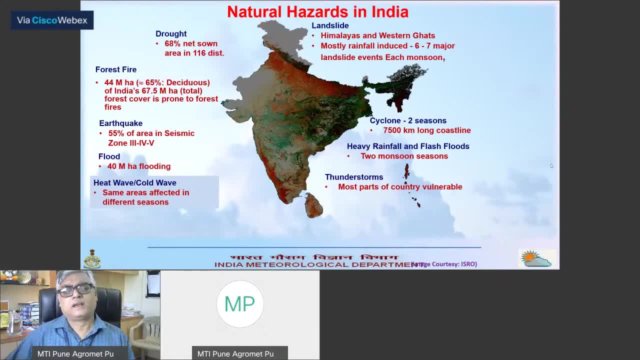 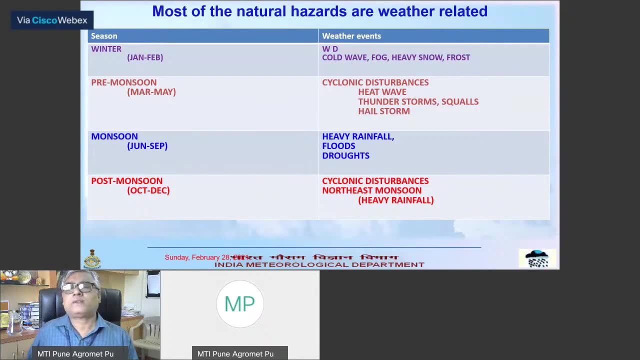 Thank you so much for your attention. Earthquake- all other are very much linked with weather condition. Most of the natural hazards are weather related and we know in India, in different season, what are the different weather events are there? Winter, it is cold wave, fog, snow, frost, pre-monsoon season heat wave. already it will start: thunderstorms, swells, monsoon, heavy rainfall. 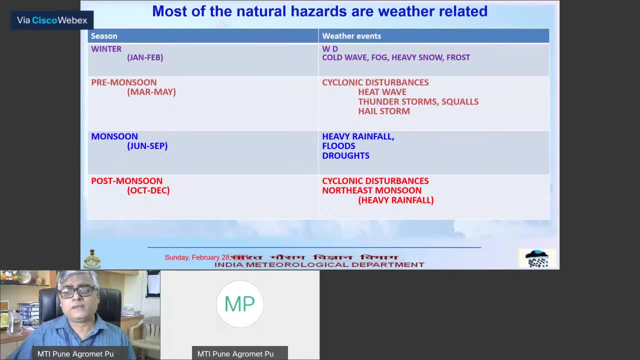 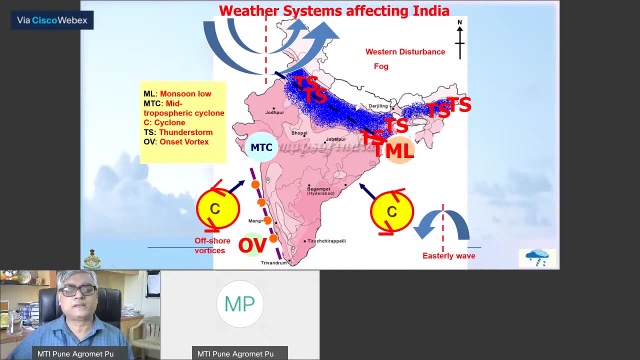 Due to monsoon, inter-seasonal variability, sometimes we get droughts at some places also, then post-monsoon cyclone, heavy rainfall. And the same thing has been schematically shown: sea stands and it is written here: sea stands for cyclone, monsoon lows, metroposphoric cyclonic circulation, offshore vortex, offshore trap, etc. monsoon trap. 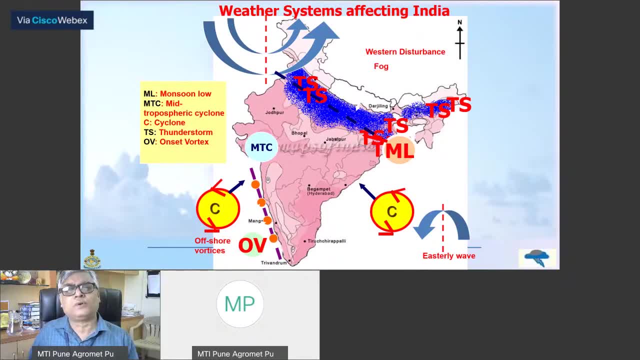 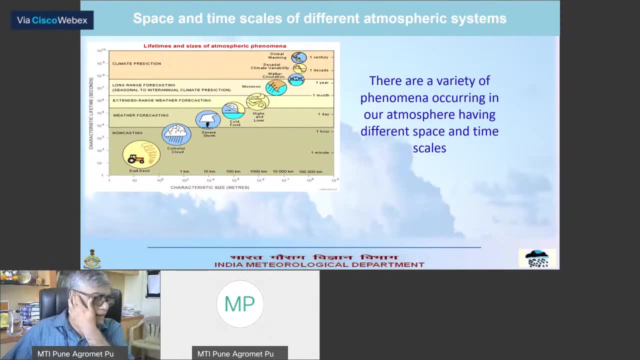 These are the things. These are the things. These are the different weather systems- This we all know- And weather system. they have different scales of time and spatial scales also. So here, actually, there are a variety of weather phenomena across different time and spatial scales. 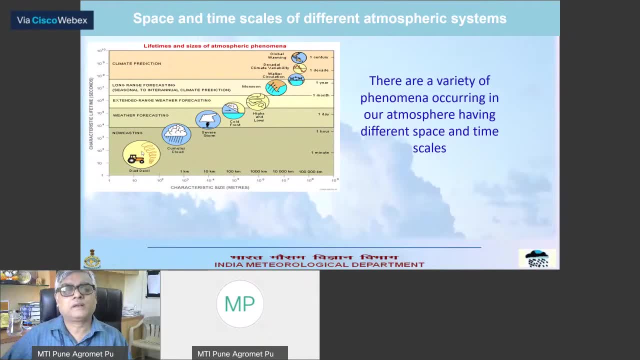 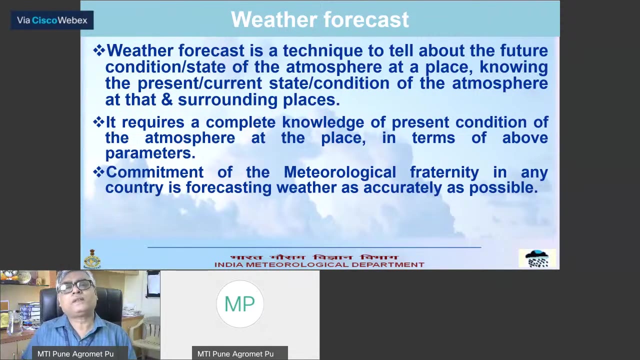 This is also a very well-known slide which shows different atmospheric phenomena. Now let us come to the topic that is weather forecast. This is a simple We can say that weather forecast is basically- it is a scientific technique to tell about the future condition or future state of the atmosphere at a place, knowing the present state of the atmospheric condition at that place, at that and also surrounding places. 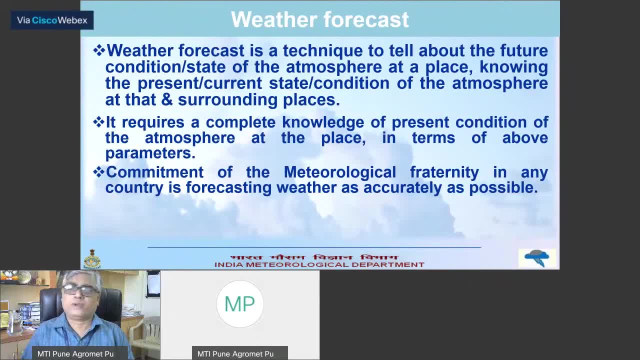 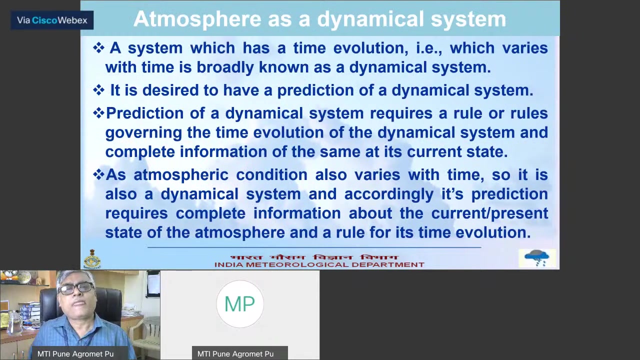 This is the weather forecast. Weather forecast requires a complete knowledge of the present condition of the atmosphere at a place in terms of those parameters which I mentioned, and we all know that meteorological fraternity in any country is forecasting weather as accurately as possible. Atmosphere as a dynamical system: dynamical system basically it refers to a system which has a time. 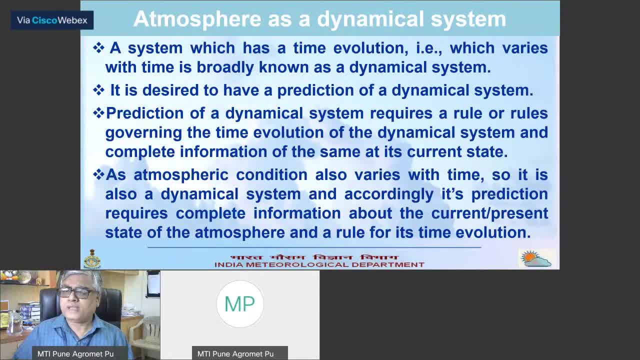 evolution means, which varies with time. so accordingly, definitely, as the atmospheric condition at a place varies with time. so therefore I can say we can definitely say that atmosphere is also a dynamical system and every dynamical system is desired to have its prediction. however, prediction of a dynamical 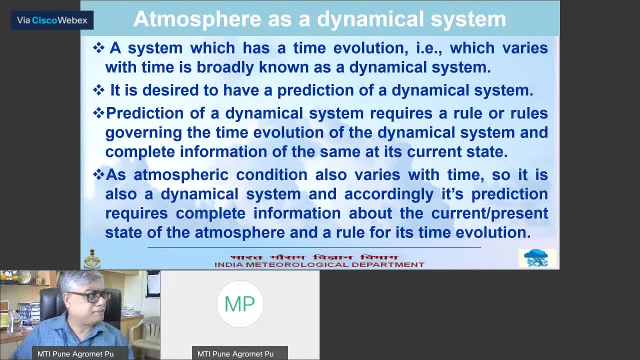 system requires two things mainly: one is the complete information of the present or current state of the dynamical system, and another one thing is required, that is, a rules which governs the time evolution of the dynamical system. So thus, that's why, that's why prediction of atmospheric condition at a place that 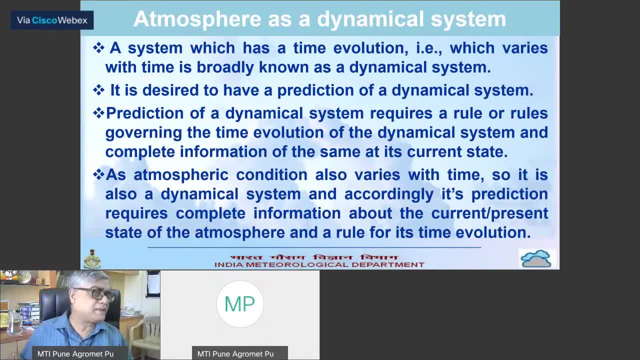 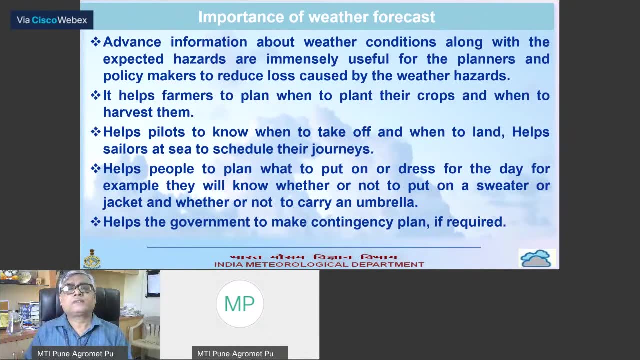 means prediction of weather at a place requires the complete knowledge or complete information about the present state of the atmospheric condition at that time, at that, at that place. Weather forecast- importance of weather focus: this is very, very, very well known. advanced information about weather condition, along with the expected hazards. 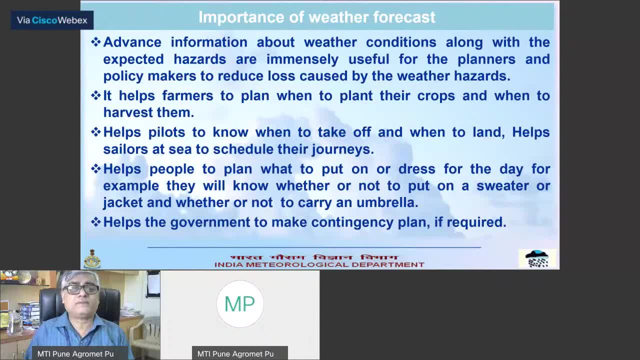 this is immensely useful for the planners and the policy makers as such, along with the advanced information about the weather condition. along with that, another one information is also very important for the planner. that is the. that is, the uncertainty in the information, then weather forecast. it helps farmers that the advance information about the weather condition helps the farmers to plan. 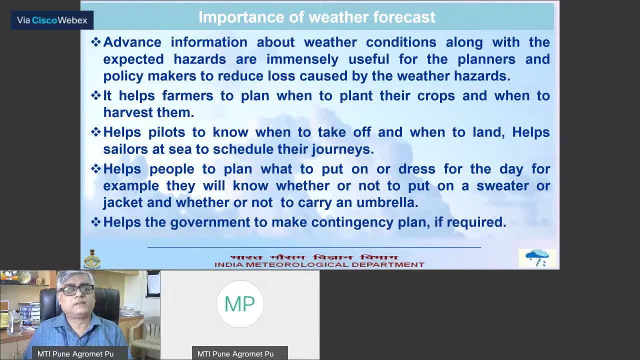 when to plant their crops and when to harvest them. it helps the pilots to know when to teacup back to land, when to land, help the seller at sea to schedule their journeys. it also helps the people to plan what to put on or dress for the day. 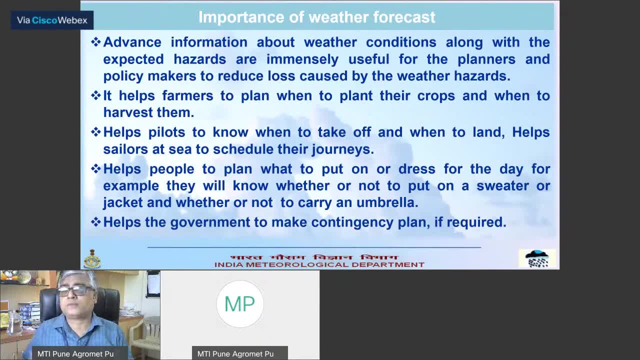 that means whether the day is hot or not, whether to put a sweater or jacket, whether to carry an umbrella, and also it helps the government to make contingency plan if required. there are many, a few of. there are many importances. i don't claim the bulleted. 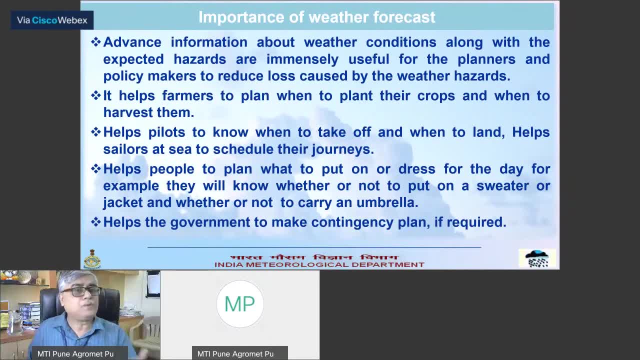 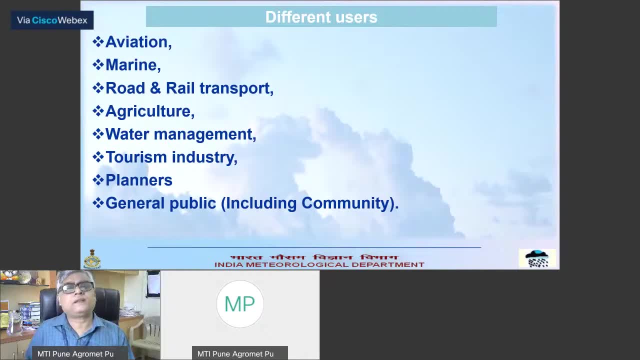 in bullet. these bullets are exhausting, a few of few only i have listed here. there are many weather forecasts have different users. air traffic as such, we can say that all transport. that's why air traffic, marine, road, rail transport, agriculture, water, tourism, planets, health, all stakeholders, hydrology sector, general public, including community. 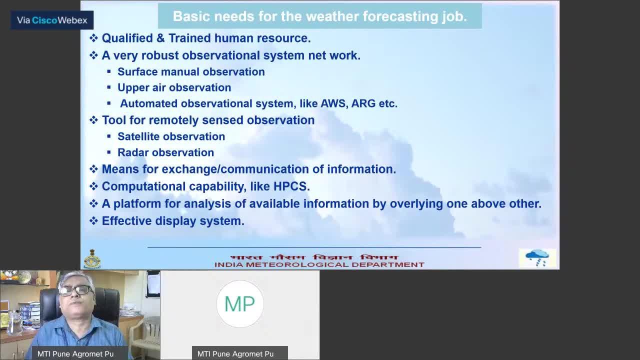 what are the basic needs for any or basic needs for the weather forecasting job? first and foremost is yes, qualified and trained human resource machine cannot do everything. a very robust observational system network consisting of surface, upper, air, automated everything tool for remotely sensed observation. also, satellite radar means for 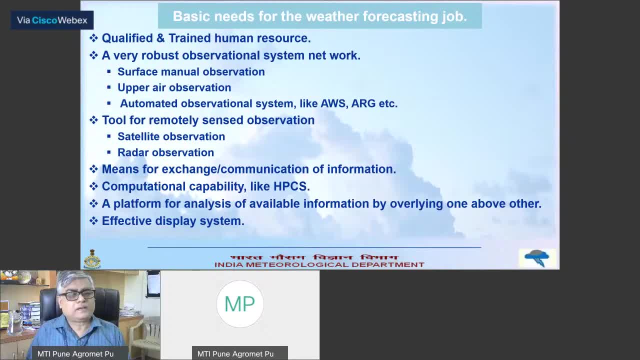 communication of information. you may- i may- have a very good quality observation, but this need to be exchanged. i cannot just keep it in my own pocket. computational capability is very, very important. computational capability, just like high power computing system. now india is having all those things i proudly i can say our mos is having. 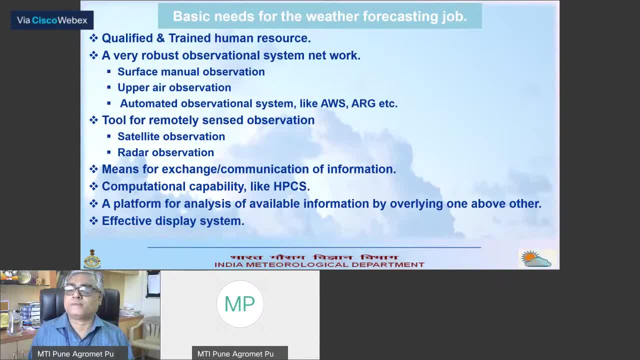 then a platform for analysis of available information, but by overlying on above another. because we are getting many informations, we are getting forecast information, we are getting observation information from different sources. all those information should be available in one platform. that is information like overlying on each other, so such systems should be also there. 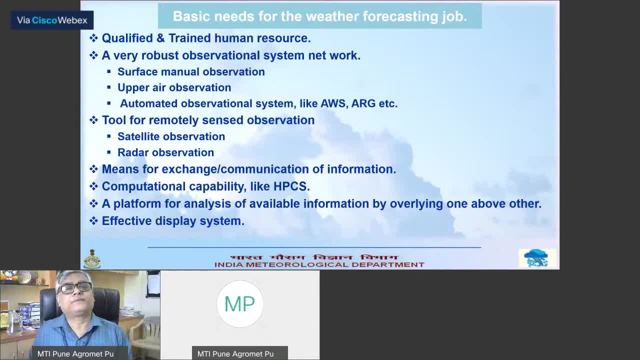 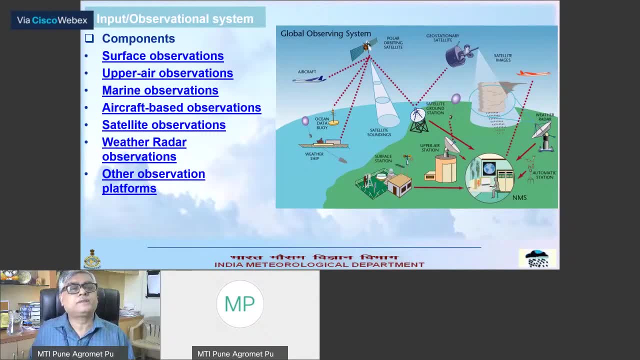 and an effective display system. these are observational system. this is a typical thing i have taken from wmo site. so these are the different components of observation system where you can see surface observation in the picture also you can see this is a typical surface observation, surface observation station. this is our national methodological service office of any country. 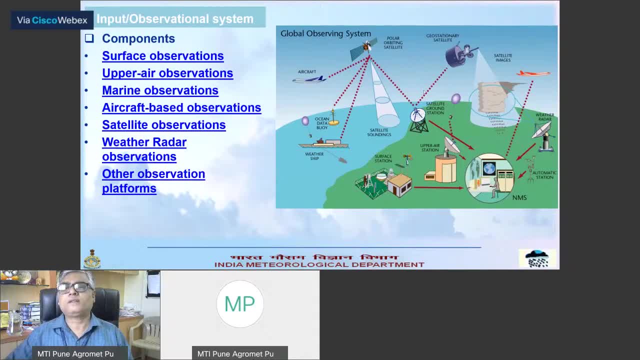 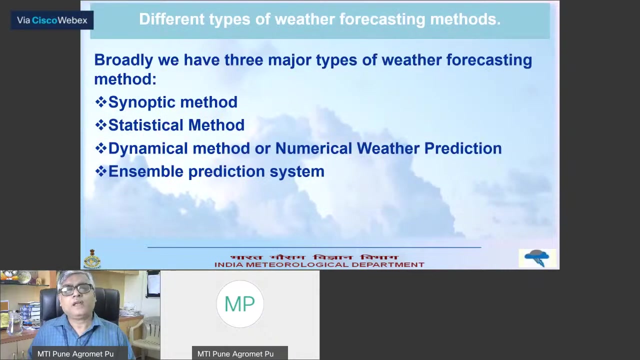 with surface stations: upper air pilot balloon- everything you can see. satellite radar- everything you can see radar, automatic weather stations- okay, everything it is there. sea weather, ocean buoy aircraft, everything. so these are the different components of observational system. now come to the weather forecasting uh method. broadly, we have three major types of 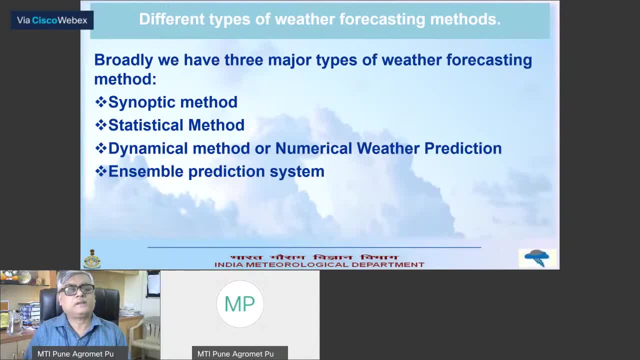 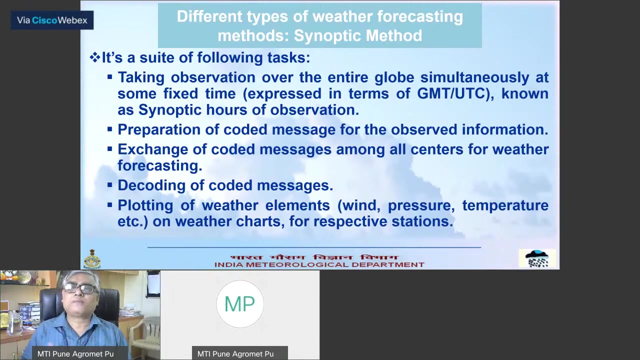 weather forecasting. one is synoptic, then statistical method. I am sorry I should have written therefore dynamical method and ensemble prediction system, but anyhow, ensemble prediction system. I can put it under this also as a sub Now in the synoptic method. actually, we all know this is a suit of different tasks. It starts from: 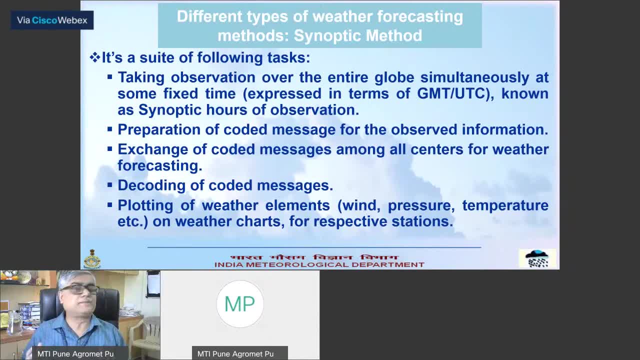 taking observation over the entire globe simultaneously at some fixed time, which we call synoptic hours of observation. Then all observed of the, then preparation of the coded messages of the observed information, exchange of the coded message among different forecasting centers. then decoding the coded messages. then plotting of the weather elements after decoding. 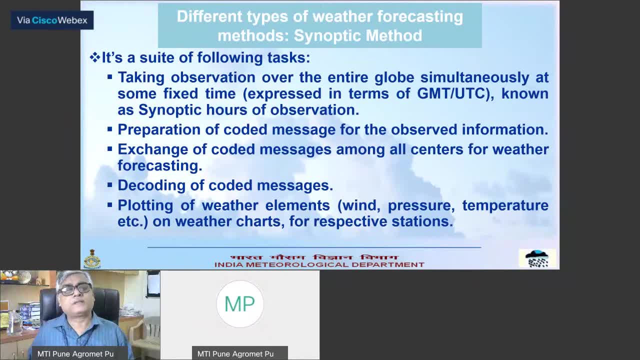 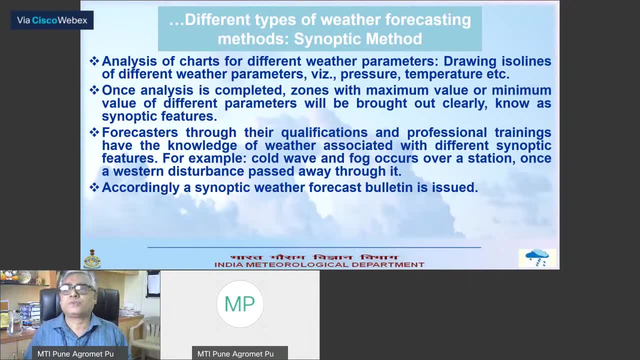 on the weather charts for respective station. Once plotting is over, then analysis of the charts of different weather parameters are done. Analysis refers to drawing of iso lines of different weather parameters, just like pressure, temperature, etcetera. When we are analyzing pressure, then we say that it is isobaric analysis. When we are analyzing temperature, that way. 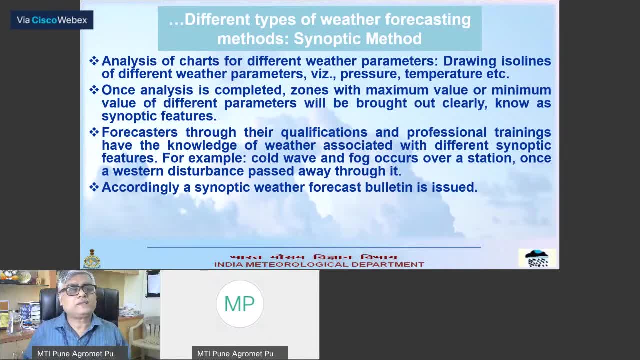 then we say it is isothermal analysis, like that. And once the analysis is completed, and if it is, if the analysis is perfect to a greater extent, Definitely we must be able to identify the zones with maximum value or minimum value of different parameters Clearly, And these are, these are our technically, we say the synoptic. 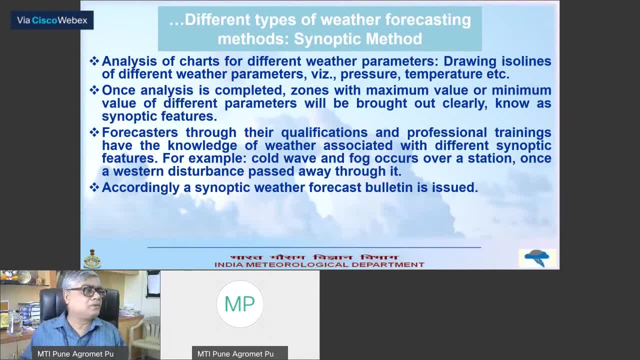 features, Synoptic features: cold area, cold warm, trough ridge, low pressure area, high pressure area- these are all synoptic features, So a good analysis must give rise to a good analysis. Synoptic features. So a good analysis must give rise to a good analysis. TheCommon is: the field analysis, Because in high pressure, in high pressure, you are focusing on the environment or the climate and you don't have to worry about the climate and you know already the climate are all large in, or you are focusing on the environment, the climate, it is in and it is in the 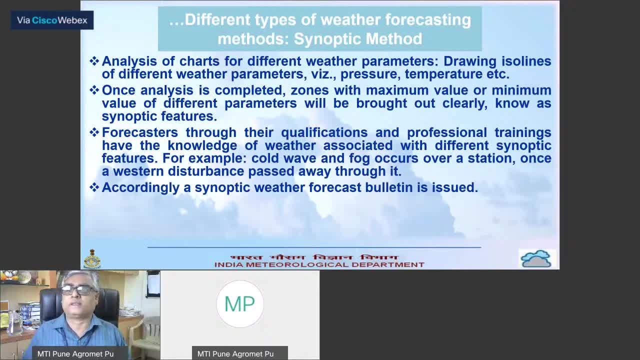 give rise to the clear identification of the synoptic features. And once the analysis is being done by the duty officers, then the analyzed chart is examined by the forecasters. and forecasters, through their qualifications and professional trainings and experience, they have the knowledge of weather associated with different synoptic. 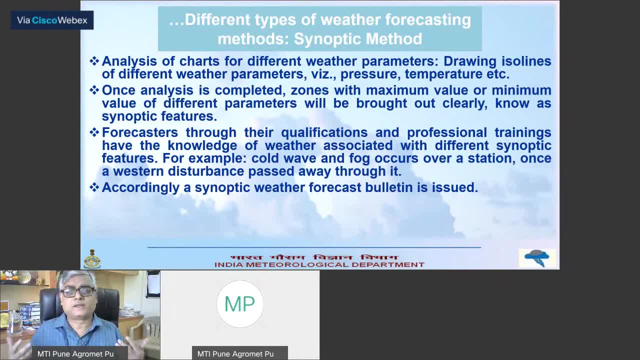 features. For example, forecasters know cold wave and fog occurs over a station once a western disturbance passed away through it. Like that there are many actually, and accordingly, using the forecasters knowledge, forecasters own knowledge and experience. forecasters issue a synoptic weather forecast. however, 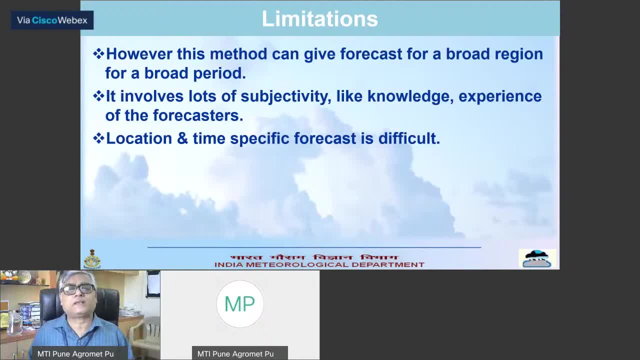 accordingly, a synoptic weather forecast bulletin is issued. So how about this method? This method has certain limitations. It is good for giving broad region for a broad period. Most important thing is it involves lots of subjectivity like knowledge, experience of 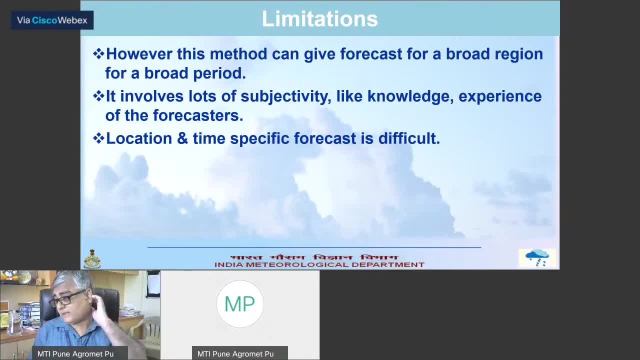 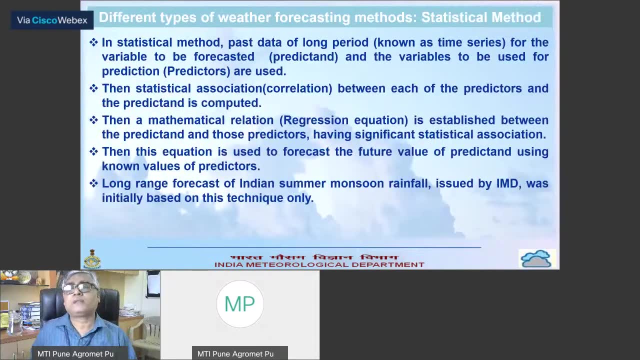 the forecasters. And another one thing is: using this method, location and time specific forecast is difficult. Next come to the another one method, that is, statistical method. In the statistical method- what I mean In the past data of long period- we say it is a time series for the variable to be forecast. 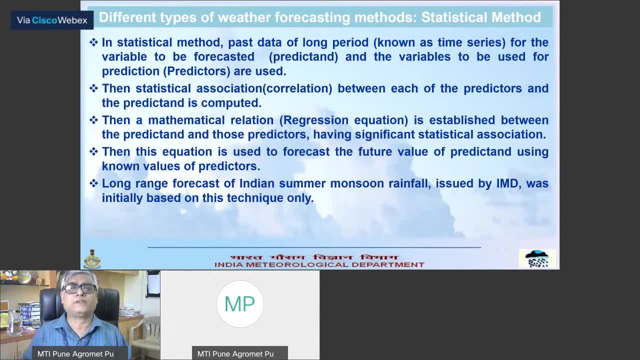 suppose if it is rainfall, then rainfall time series. we use The variable to be forecast, we call- we know that we call it predict- and the variables to be used for the prediction each time series. also. we are having this time two time this. 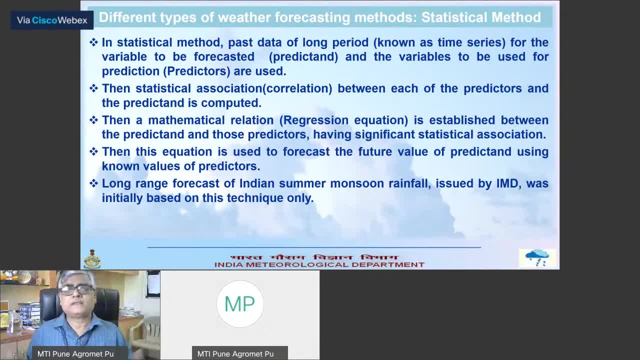 two or more time series we are using. Then statistical association, that is, correlation between each of the predictors and the predictor, is computed. Then regression equation, a mathematical relation, is established. we call it regression equation. It may be linear, it may be multiple, it may be simple, it may be multiple, it may be linear. 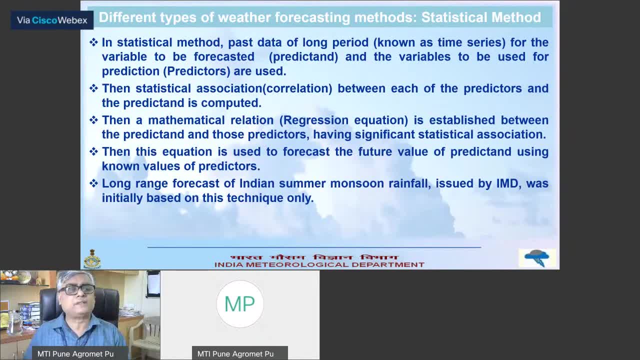 non-linear, whatever it may be, is established between the predictor and the. those are predictors, All predictors, not all predictors. having predictors having significant correlation, Then this equation it is used for forecast the future value of the predictor. This is a quite well-known and very popular method also, and we all know that long-range. 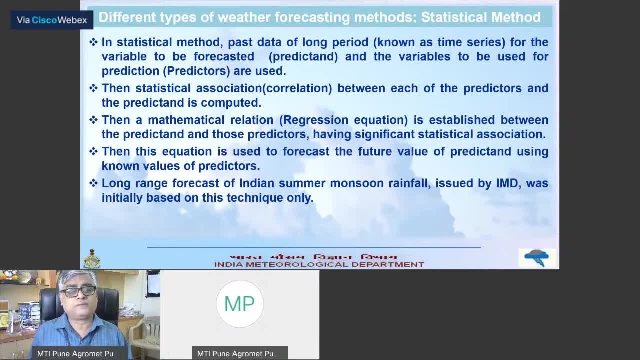 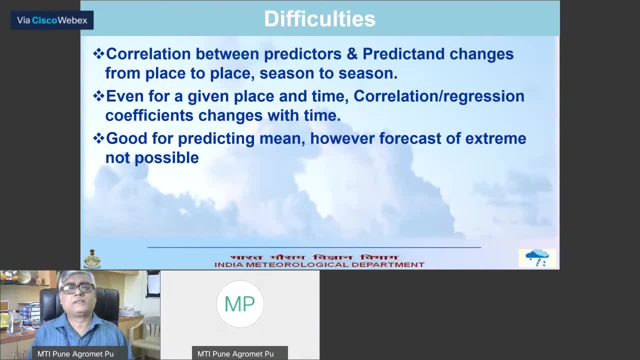 forecast of Indian summer monsoon rainfall issued by IMD was initially based on this statistical technique only. However, this method is also having some difficulties. First of all, this correlation between the predictors and predictor. it changes go on changing from place to place, season to season, even for a given place and time correlation. 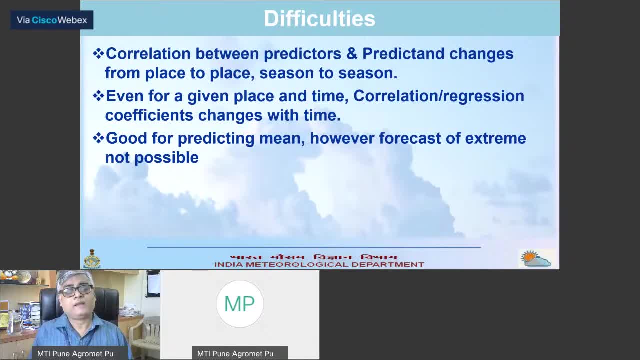 and regression coefficient. it changes with time. And another one thing: statistical prediction. it is good for predicting mean. however, in case of extreme weather it may fail, fail and most important thing, is that reason of the exploding, the reason of the failure, may be very, very difficult, rather impossible. 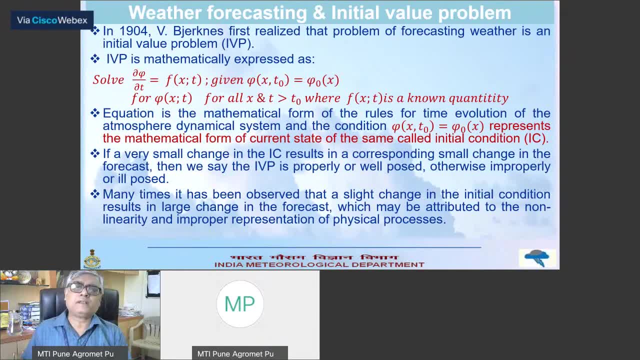 Then comes to now, before starting the numerical prediction. Now, before starting the numerical prediction, I will just try to inform that weather forecasting and the initial value problem. In 1904, Barton is first realized that the problem of forecasting weather is an initial 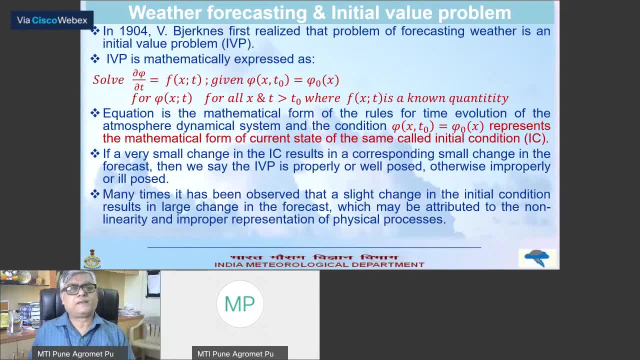 value problem. Initial value problem is mathematically. it is expressed as solving a partial differential equation. on the left-hand side, first order time derivative of an unknown function is there. On the right-hand side, a known function of space and time is there. 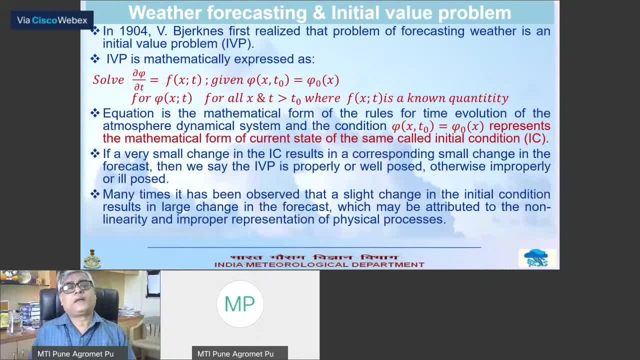 And, along with that, that value of the unknown function at the initial time, that is, current time, at all points are given. it is available with us And what is our task? task is to find out the value of the unknown function at all future. 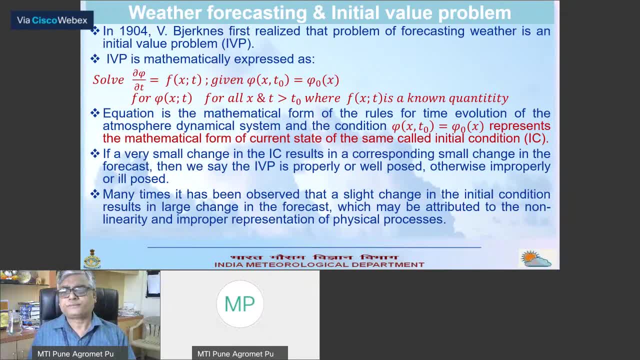 time, at all the points. This is actually, mathematically we say it is an initial value. problem, Equation, whatever equation, this equation, Delphi, this first equation, this equation is nothing but the mathematical form of the rules which I have mentioned in the slides. 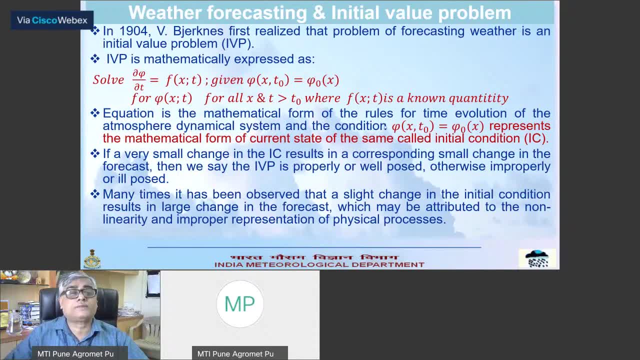 of dynamical system, rules for time, evolution of the atmosphere dynamical system And the given condition. this condition is nothing but the mathematical form of the current state of the dynamical system, the atmosphere dynamical system. we call it initial condition. 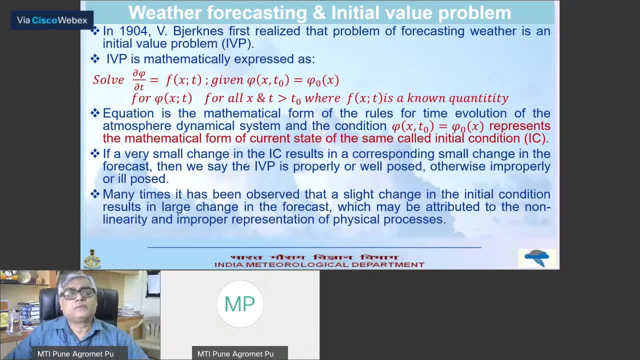 If a very now, now, one thing we can do, that suppose I am having an initial condition, using that initial condition I am solving it, And when I am solving it for a given point, let us say, then I am having different value. 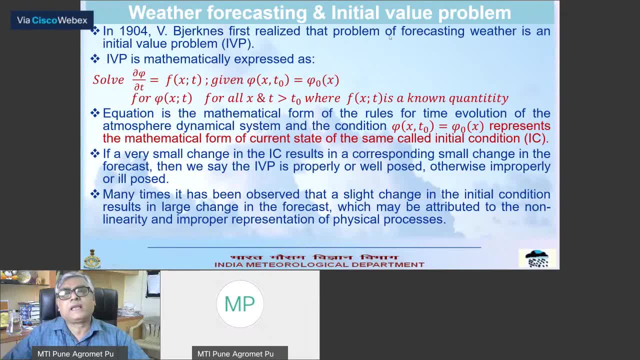 of this unknown function. Okay, So if I have a given function at different time, then I can draw a graph: y-axis value of the unknown function at different time and x-axis all future time. And if I plot it and after the after joining the plotted points, I will get a graph. 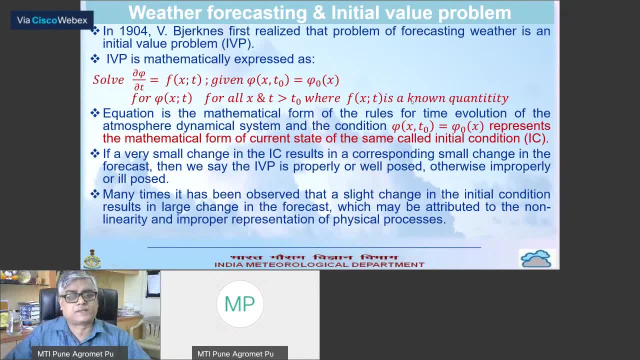 This graph, we will say it is a forecast trajectory. forecast trajectory. Now, if I change very little the initial condition, Okay, The initial condition. technically we call it a small perturbation in the initial condition. And if it results similar small change in the forecast, then we say this initial value. 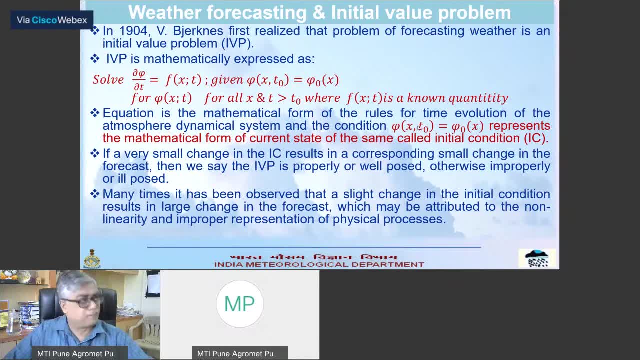 problem is well posed or properly posed. but if it doesn't happen, that means if due to a slight change in the initial condition, then we say this initial value problem is well posed or properly posed. But if it doesn't happen, If there is a large change in the forecast, then we say this initial value problem is. 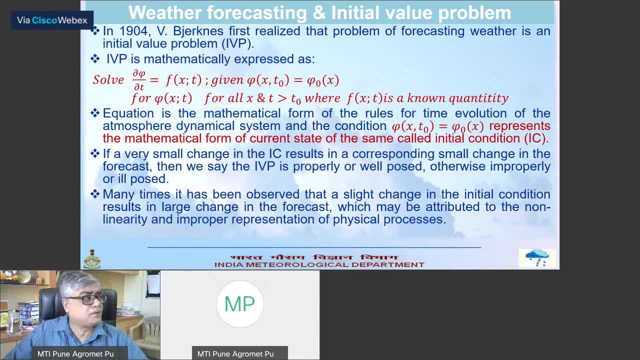 improperly posed or ill-posed. that is not well posed And many times it has happened. also, it has been observed that a slight change in the initial condition results in large change in the forecast, and this may be attributed to the non-linearity and impropriety. 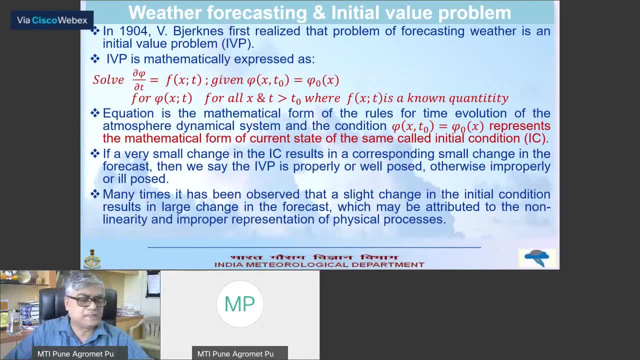 Okay, So the non-linear term- The non-linear term is a word, representation of the physical process In the atmosphere. in the atmosphere, whatever governing equations are there, that is, this type of equations are there. On the right-hand side, there are terms which are expressed as a product of two dependent 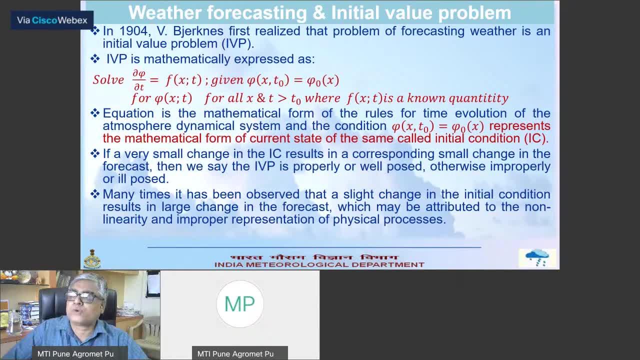 variables, Such terms, we call it non-linear terms, And those non-linear terms are representative of the physical process. Okay, Okay, the non-linear effect or non-linearity of the atmosphere. of course, our atmosphere is non-linear, and so that's why it is this change, this, uh, this, that means this ill-posedness of the initial 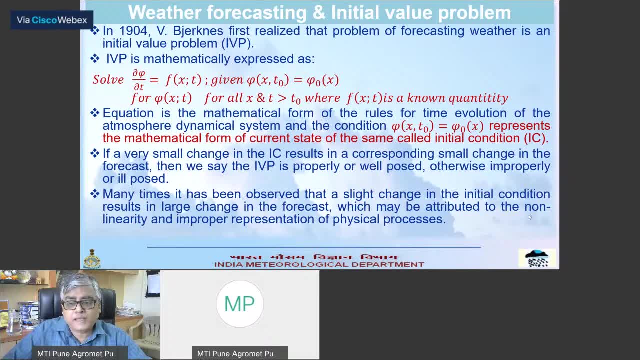 initial value problem may parts may be attributed to a greater extent to the non-linearity that is, presence of such non-linear terms in the governing equations and also improper representation of physical processes in the atmosphere. there are many physical processes are there which we, which we could not represent perfectly in mathematically, in mathematical terms. 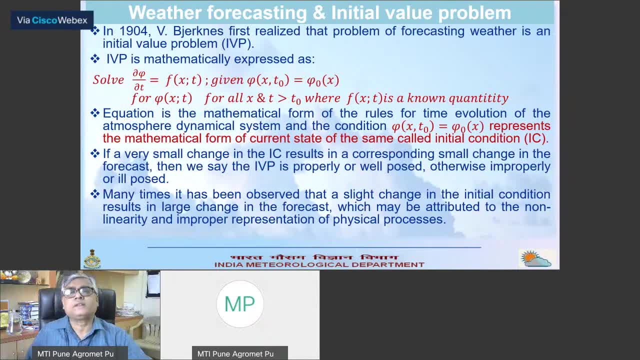 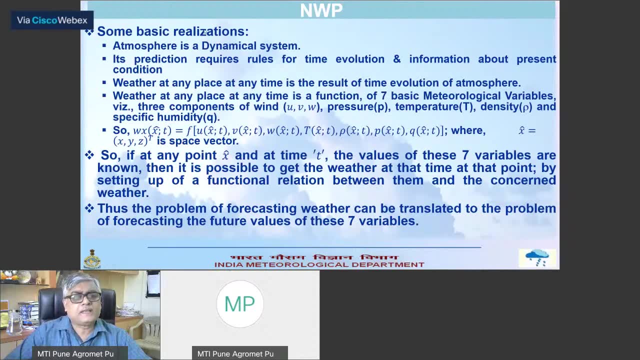 so this is also- this may also be one of the reason in the nwp. there are certain basic realization is there that atmosphere is a dynamical system. accordingly, its prediction requires rules for time evolution. most important realization is whether, at any place at any time, is that result of time? okay, that is. 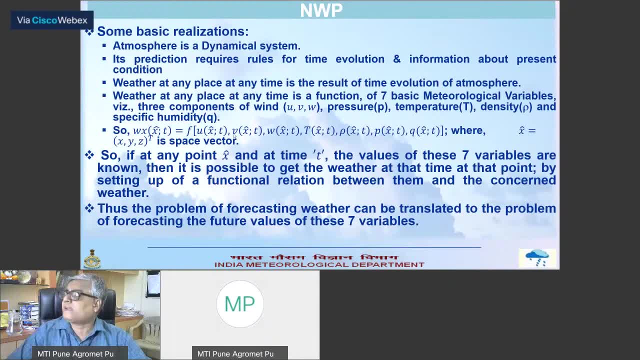 not this one. whether, at any place, at any time, is a function of some basic meteorological parameters, which are your wind pressure, temperature, humidity, density, etc. and mathematically we say whether wx is, whether x cap. this is the spatial point, three dimensional spatial point. whether at any time it is a function f stand function of. 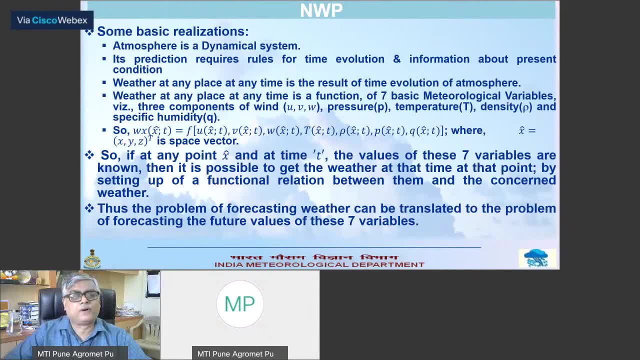 all these variables, all these variables. so, therefore, if i know, if i know the value of the seven parameters at a given time, at a point, then it is possible to find out the weather at that point, at that time. so, therefore, the problem of forecasting weather has now been translated. 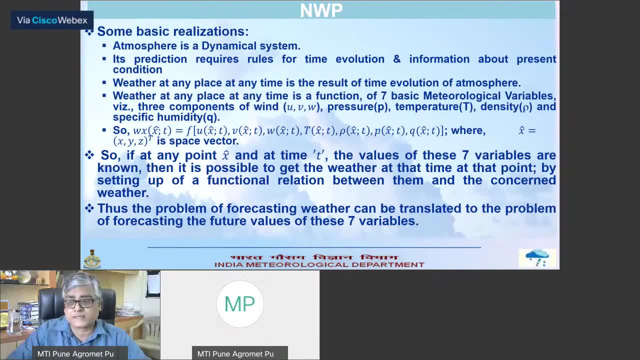 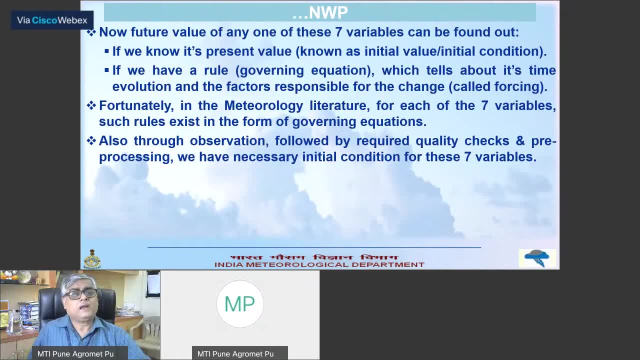 can be translated to the problem of forecasting the future values of these seven variables. now, few very important things now tell me actually what is the future value of weather? future value of any one of these seven variables can be found out if we know their present value. that means if we have the initial, if we know the initial condition for each of them, and also if we 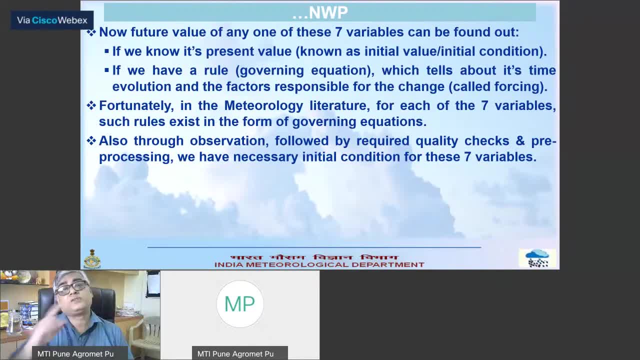 have a rule for the time evolution of each of these seven parameters, which we call governing equation. fortunately, we are fortunate enough. fortunately, in the metallurgy literature for each of these seven variables such rules are available and fortunately, through a robust observational system followed by required quality checks and pre-processing, we have necessary. 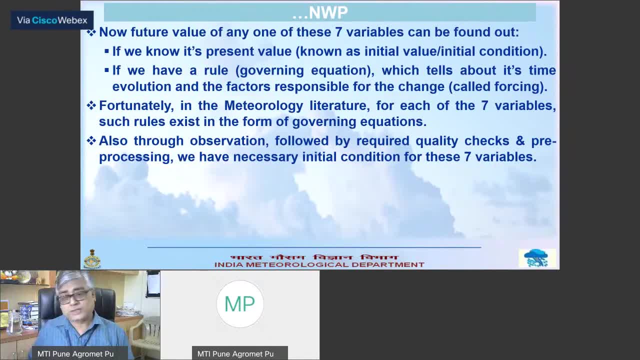 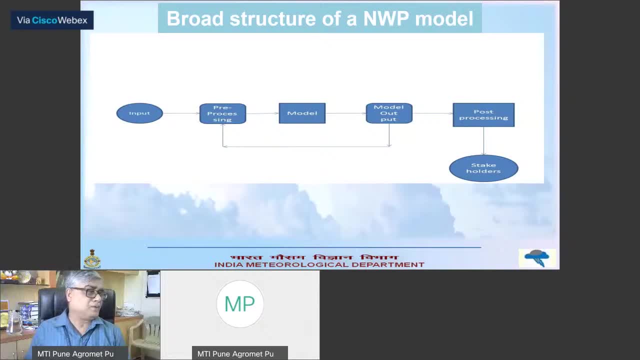 initial condition for these seven variables. so, theoretically or in principle i: in principle, nwp should be able to provide time and location. specific, for it is a generic, broad structure of any nwp model, every nwp model, there will be one, an input. those inputs need to be: 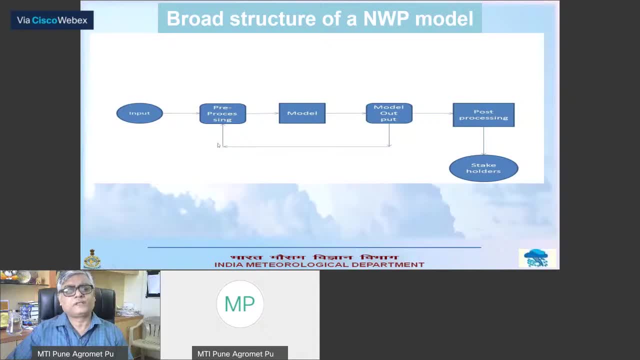 pre-processed. so there will be a pre-processing unit, reprocessing unit, then pre-processed initial condition goes to the model. in the model, those governing equations are integrated forward with respect to time numerically: numerically for each and every regularly spaced grid points in grid points and a future value at every time state for all these. 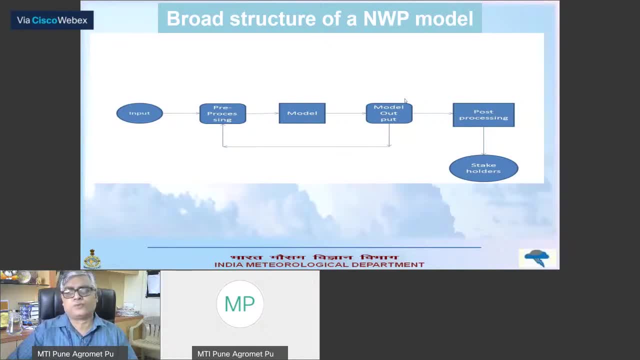 seven variables which are nothing but your model of time output. this model output we cannot provide directly to the stakeholders as it has a very little use by the stakeholders- direct value. so therefore it needs also post processing, post processing and also model output. it also goes to the pre-processing for the next. 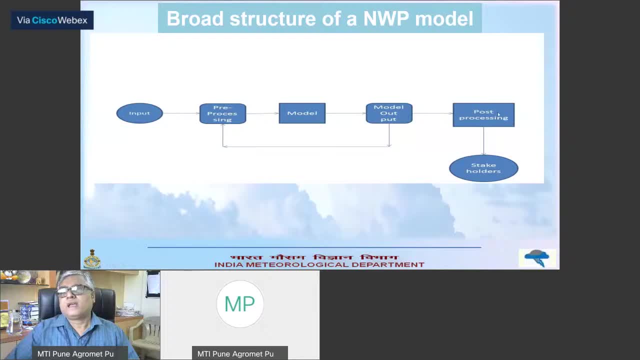 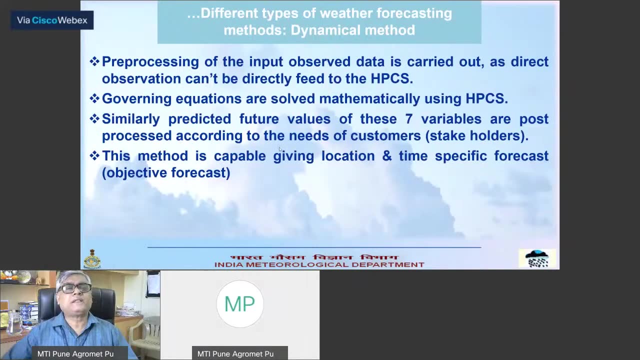 next time, next time and after post processing it goes to the stakeholders. so that is, this is in the pre-processing because of the input observed data in the pre-processing of the input observed data is carried out as direct observation- cannot directly fit to the htcl. so whatever i told, the same thing is. 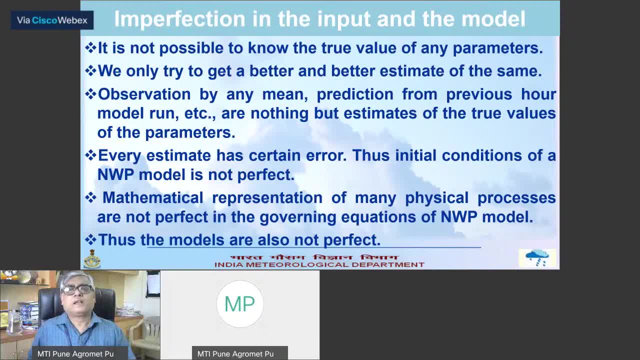 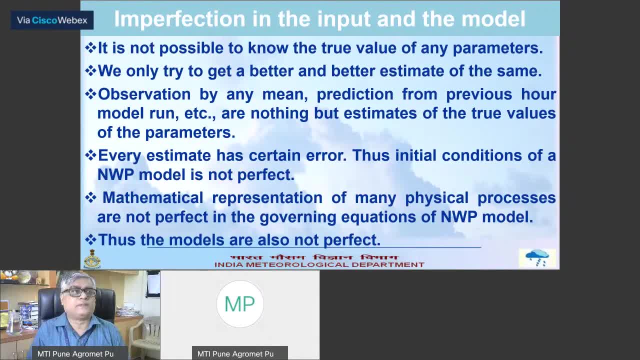 not perfect. it is not possible to know the true value. it is not possible to know the true value, it is not possible to know the true value of any parameters, of any parameters, of any parameters. many times we think that, whatever we are, many times we think that whatever we are. 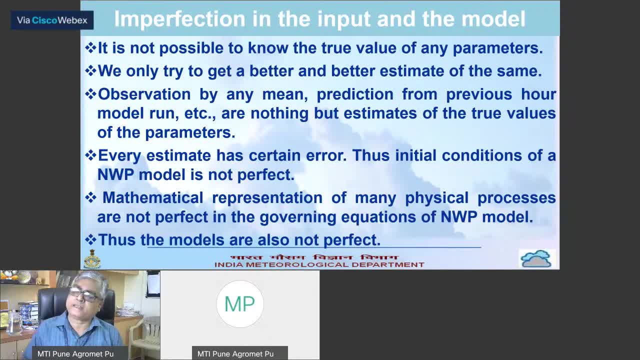 many times we think that whatever we are observing, that is the true value of that observing. that is the true value of that observing. that is the true value of that parameter at that place at that time. it parameter at that place at that time. it parameter at that place at that time. it is not so. 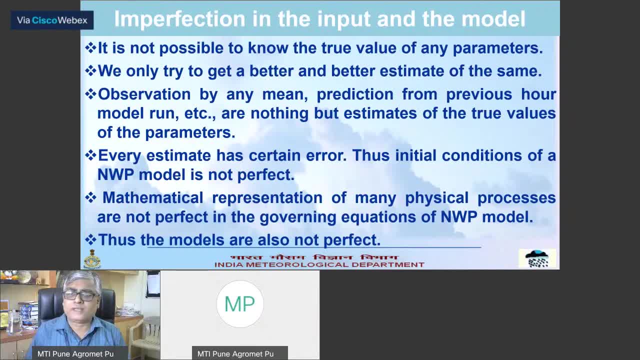 is not so. is not so because true value we cannot, because true value we cannot, because true value we cannot. we cannot find out. we cannot find out, we cannot find out. we only try to get a better and better. we only try to get a better and better. 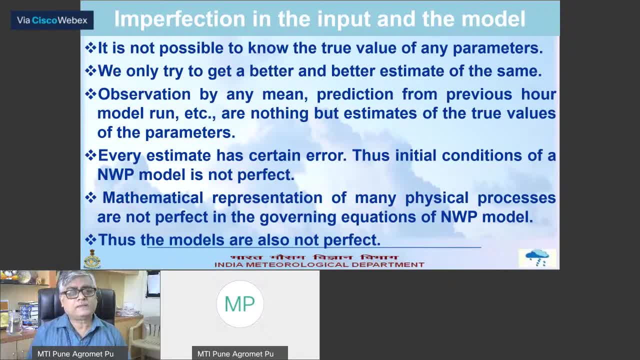 we only try to get a better and better estimate of the true value, estimate of the true value, estimate of the true value, observation, observation, observation by, by, by, uh, uh, uh, any mean, any mean, any mean, just like, just like, just like, direct figure, man-made observation, or. 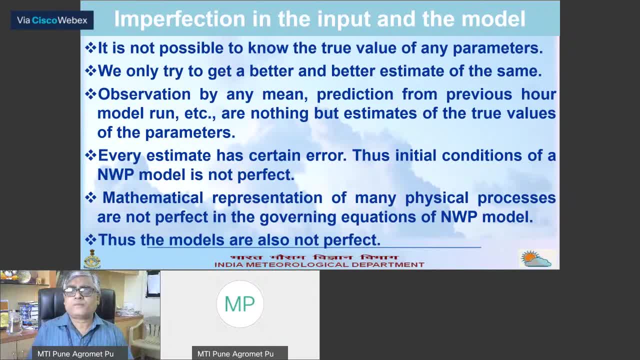 direct figure man-made observation or direct figure man-made observation or machine-made observation. machine-made observation or machine-made observation, or prediction from previous our model run, prediction from previous our model run, prediction from previous our model run. these are all nothing but the. these are all nothing but the. 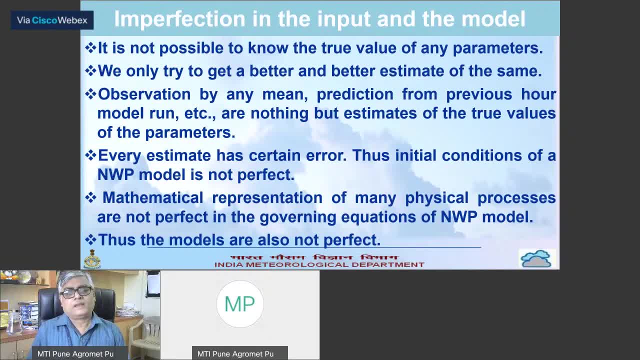 these are all nothing but the estimates of the true values, of the estimates of the true values, of the estimates of the true values of the current, current, current, and and. and. statistical theory tells us that statistical theory tells us that statistical theory tells us that every estimate has certain error. 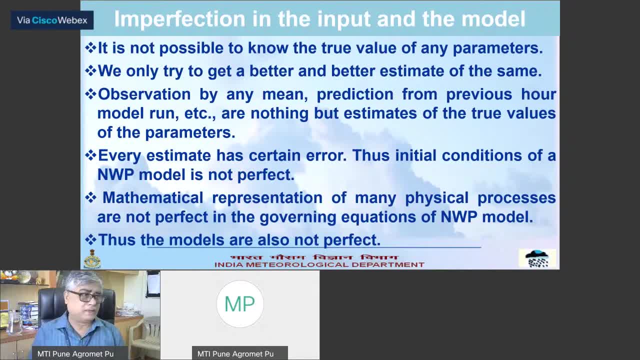 every estimate has certain error. every estimate has certain error. so thus, whatever initial condition, we so thus, whatever initial condition, we so, thus, whatever initial condition we are providing to the model even after, are providing to the model even after, are providing to the model even after pre-processing also. 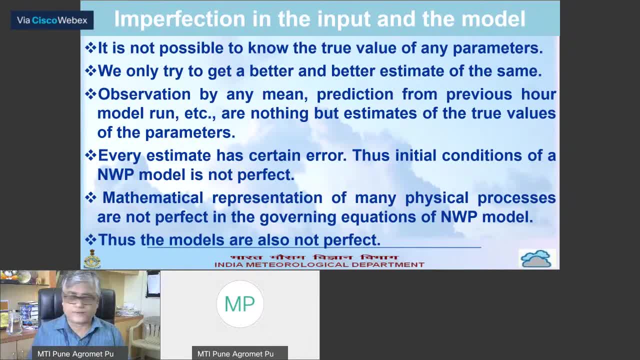 pre-processing also. pre-processing also. we cannot say with guarantee, that is 100. we cannot say with guarantee, that is 100. we cannot say with guarantee, that is 100, it is perfect, that is 100, it is perfect, that is 100, it is perfect, that is 100 correct. 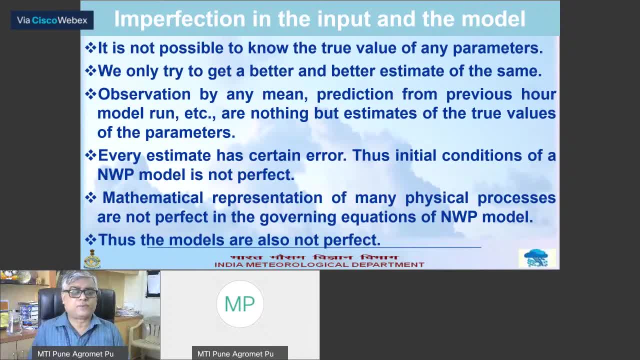 correct, correct. another one thing mathematical, another one thing mathematical, another one thing mathematical: representation of many physical representation of many. physical representation of many physical processes are not perfect in the processes, are not perfect in the processes, are not perfect in the governing equations as i, governing equations as i. 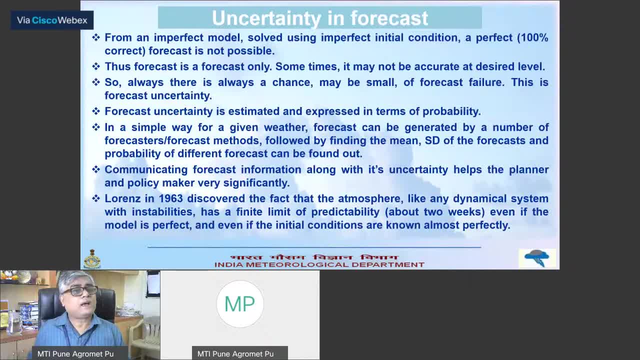 governing equations, as i model is also not perfect, model is also not perfect, model is also not perfect. so thus, so, thus, so, thus, thus, thus, thus, from an imperfect model, from an imperfect model, from an imperfect model, solving solved using imperfect initial solving, solved using imperfect initial solving, solved using imperfect initial condition. 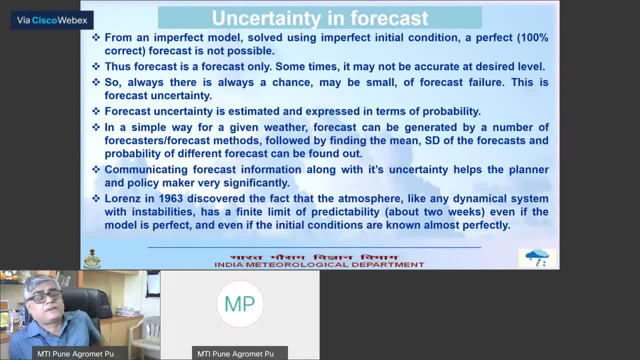 condition. condition: a perfect forecast, a perfect forecast, a perfect forecast. desiring a perfect focus is too much. it desiring a perfect focus is too much. it desiring a perfect focus is too much. it is not possible. basically, theoretically is not possible. basically, theoretically is not possible. basically, theoretically it is not possible. 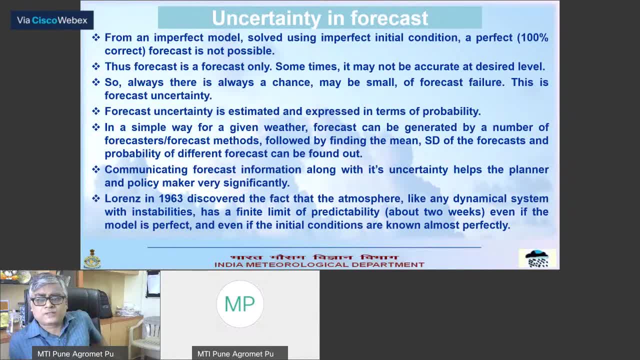 it is not possible. it is not possible. thus, thus, thus, forecast is forecast, only forecast is forecast, only forecast is forecast, only every forecast contains certain amount, every forecast contains certain amount, every forecast contains certain amount of error, certain amount, ever always there, of error, certain amount, ever always there. 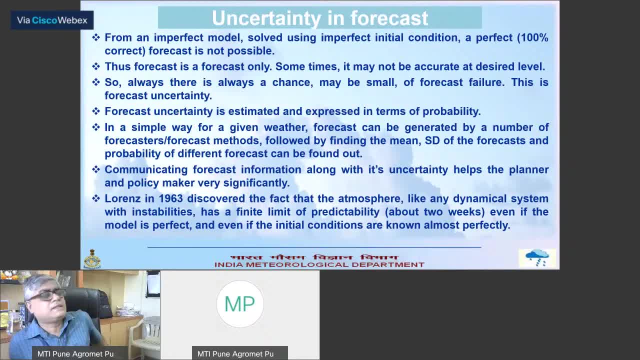 of error, certain amount, ever, always, there is a chance, is a chance, is a chance, maybe small of forecast period. this is maybe small of forecast period. this is maybe small of forecast period. this is nothing but forecast failure means nothing but forecast failure means nothing but forecast failure means forecast error. 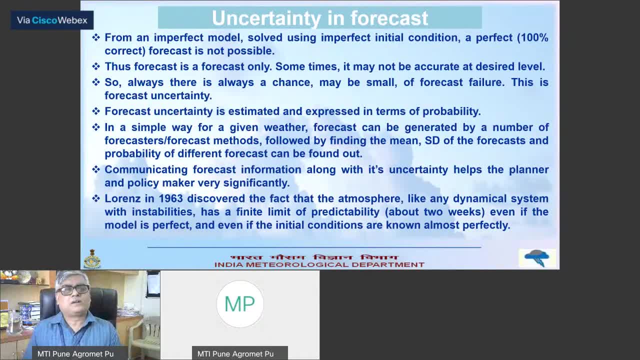 forecast error. forecast error beyond the tolerance limit. this is your. beyond the tolerance limit. this is your. beyond the tolerance limit. this is your. this is our forecast uncertainty. this is our forecast uncertainty. this is our forecast uncertainty, forecast uncertainty is estimated and forecast uncertainty is estimated and forecast uncertainty is estimated and expressed in terms of probability. 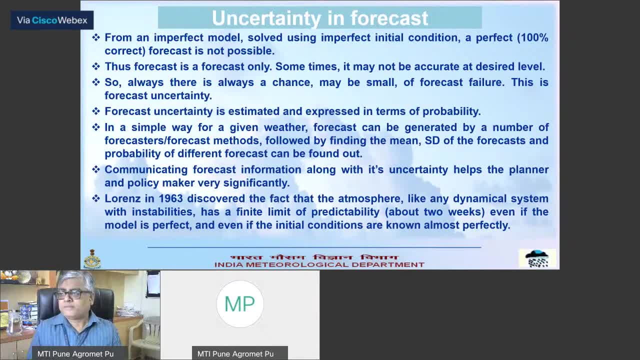 expressed in terms of probability, expressed in terms of probability. so therefore, one thing is very clear. so, therefore, one thing is very clear. so, therefore, one thing is very clear: if for a given weather phenomena, if for a given weather phenomena, if for a given weather phenomena at a given time, at a given place. 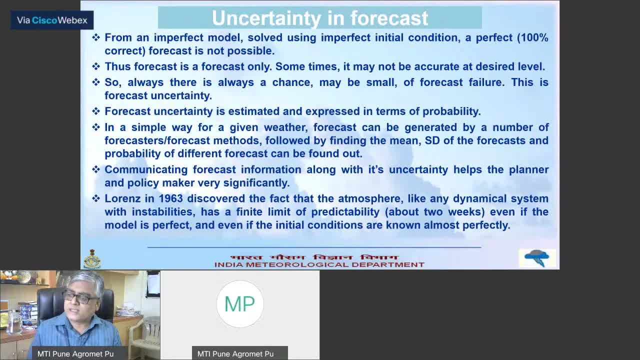 at a given time at a given place. at a given time, at a given place, using a given initial condition, using a given initial condition, using a given initial condition, using a given model. i cannot expect more using a given model. i cannot expect more using a given model. i cannot expect more than one focus. i will have only one. 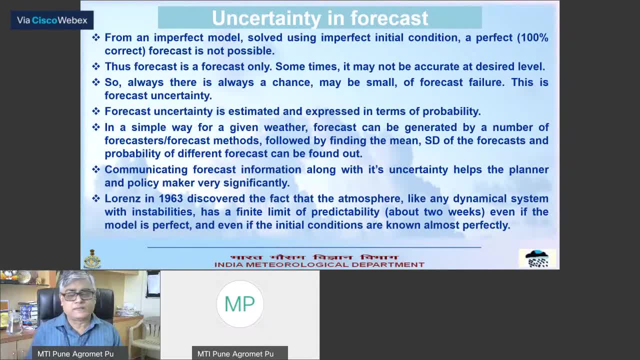 than one focus. i will have only one than one focus. i will have only one focus, focus, focus. and that forecast- we all know this is and that forecast- we all know this is, and that forecast- we all know this is called a deterministic focus. so therefore, called a deterministic focus. so therefore, 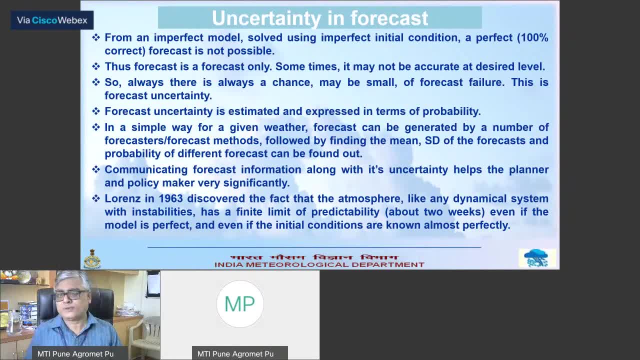 called a deterministic focus. so therefore, we cannot do, we cannot do, we cannot do. any statistics on that, it is not possible. any statistics on that it is not possible. any statistics on that it is not possible. for that, for that we should have. for that, for that we should have. 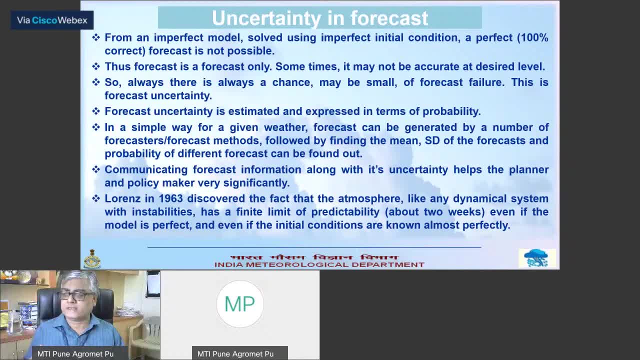 for that. for that we should have number of focus, number of focus rather i number of focus, number of focus rather i number of focus, number of focus, rather, i can say it is a sample of focus, can say it is a sample of focus, can say it is a sample of focus. if i have a sample of focus then i can 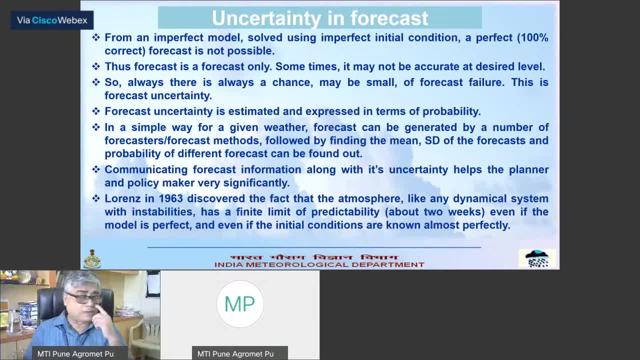 if i have a sample of focus, then i can. if i have a sample of focus, then i can talk of many things, talk of many things, talk of many things. i can talk about the mean i can talk. i can talk about the mean i can talk. i can talk about the mean i can talk, talk about the standard division. even i. 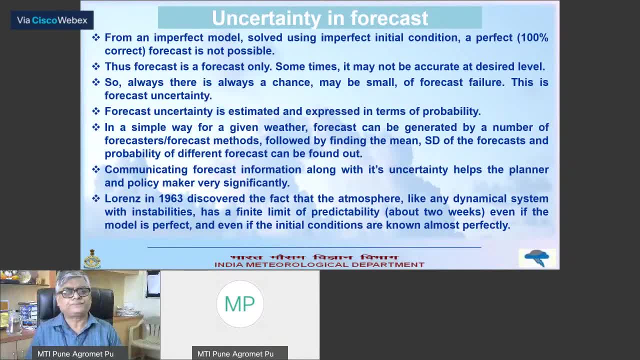 talk about the standard division, even i talk about the mean. i can talk about this probability distribution function, about this probability distribution function, about this probability distribution function also, also also. so that is also in a simple way for a. so that is also in a simple way for a. 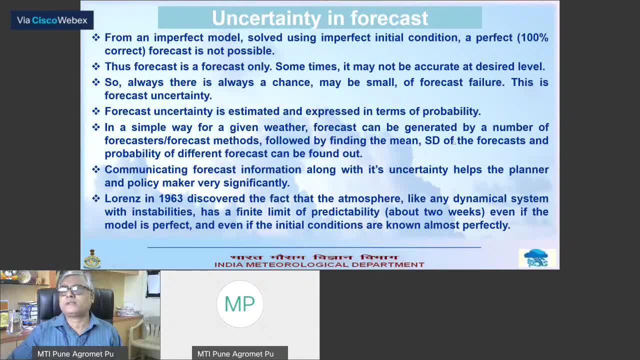 so that is also in a simple way: for a given weather, given weather, given weather forecast. given weather forecast can be forecast, given weather forecast can be forecast, given weather forecast can be generated by a number of forecasters, or generated by a number of forecasters, or generated by a number of forecasters, or forecasting method. 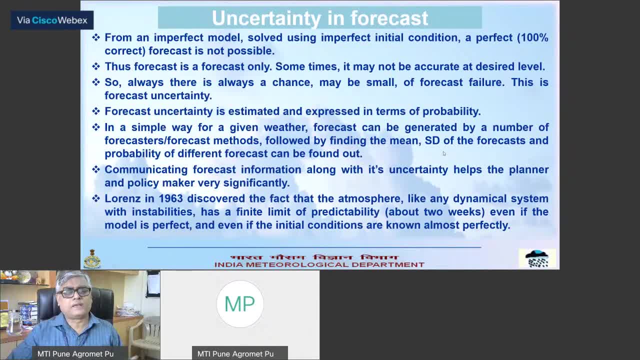 forecasting method. forecasting method, followed by finding the main standard of, followed by finding the main standard of, followed by finding the main standard of what i told, what i told, what i told. communicating forecast information along communicating forecast information along. communicating forecast information, along with its uncertainty, helps the planner. 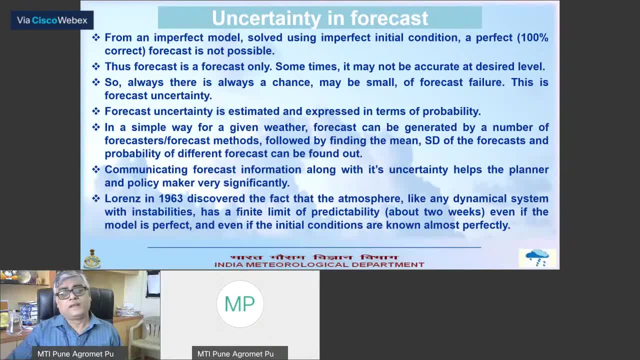 with its uncertainty, helps the planner with its uncertainty, helps the planner and policy makers very significantly, and policy makers very significantly and policy makers very significantly. another one important thing. that is another one important thing. that is another one important thing that is lawrence in 1963 discovered. 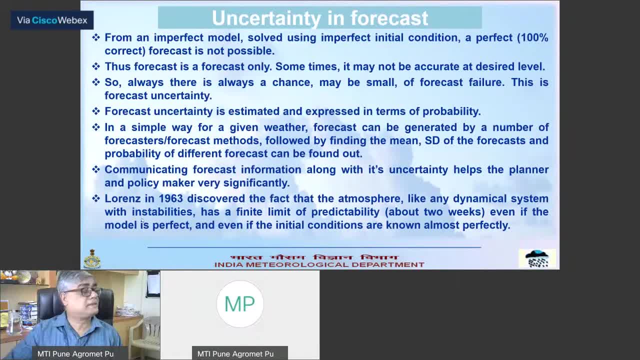 lawrence in 1963 discovered. lawrence in 1963 discovered the fact that the atmosphere like any, the fact that the atmosphere like any, the fact that the atmosphere, like any dynamical system with instabilities, dynamical system with instabilities, dynamical system with instabilities- has a limit of predictability. that means: 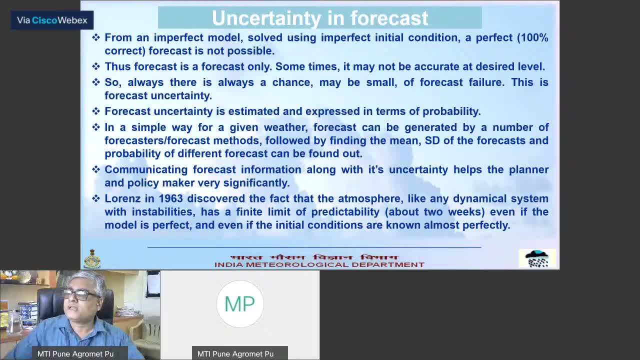 has a limit of predictability. that means has a limit of predictability. that means beyond certain period. we can't expect beyond certain period. we can't expect beyond certain period. we can't expect the correct forecast okay within certain. the correct forecast okay within certain. the correct forecast okay within certain tolerance limit. it is not possible as a 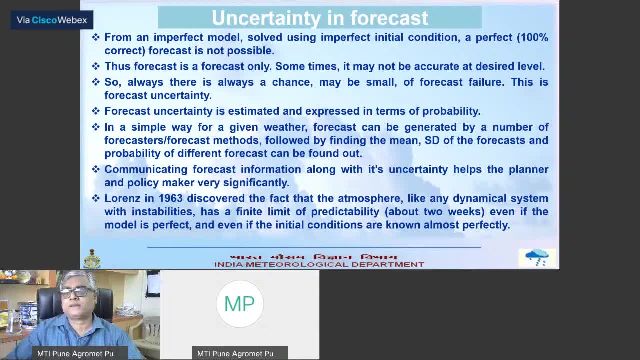 tolerance limit. it is not possible as a tolerance limit, it is not possible as a certain certain, certain finite limit of predictability. he has finite limit of predictability. he has finite limit of predictability. he has properties of two weeks, even if the properties of two weeks, even if the 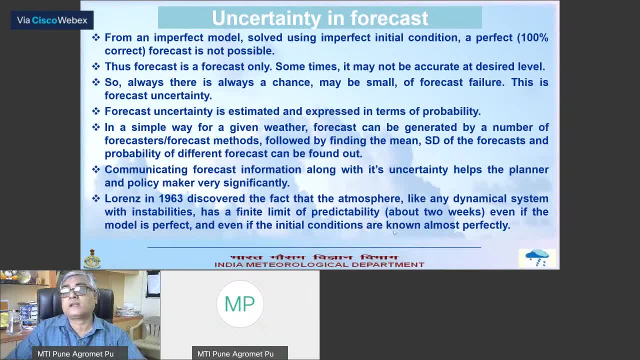 properties of two weeks, even if the model is perfect and even if the initial model is perfect and even if the initial model is perfect and even if the initial conditions are, conditions are conditions are known almost perfectly theoretically. it known almost perfectly theoretically, it known almost perfectly theoretically. it is called deterministic chaos because our 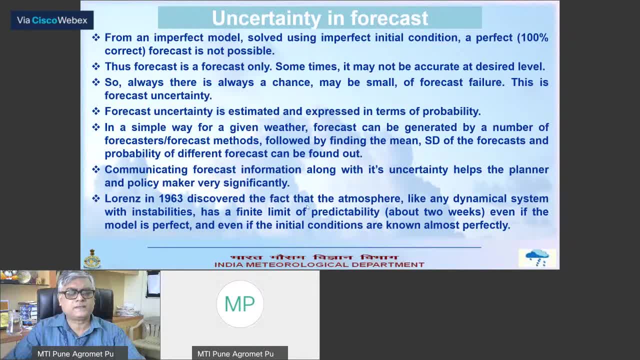 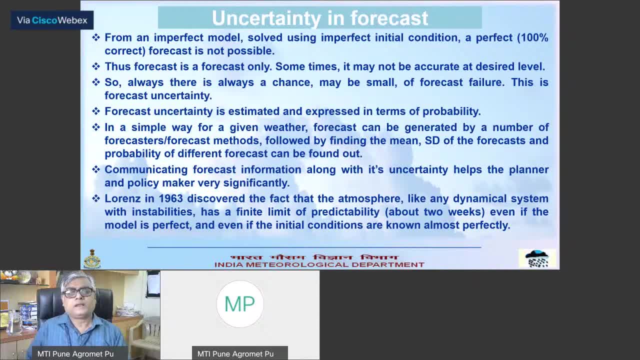 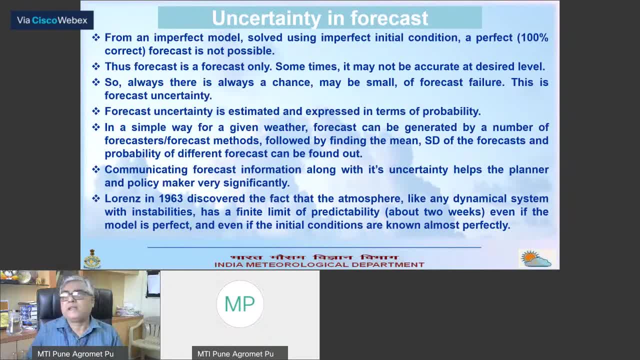 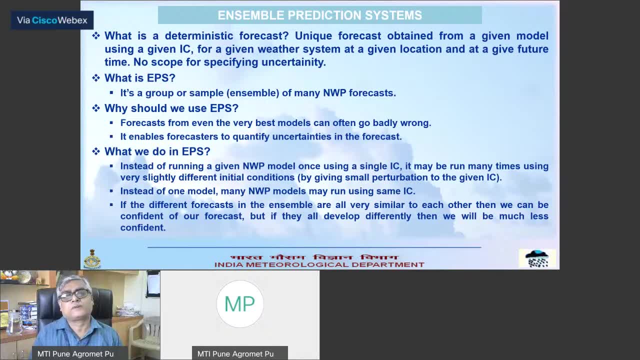 arrangement, arrangement of providing the information about the, of providing the information about the, of providing the information about the uncertainty in the focus, and this uncertainty in the focus and this uncertainty in the focus, and this gives rise to, gives rise to, gives rise to another one forecast system, that is: 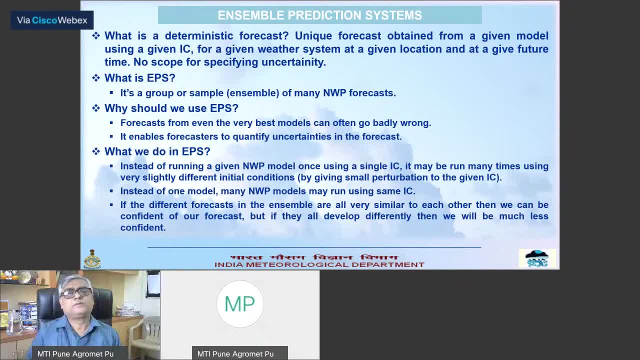 another one forecast system. that is another one forecast system. that is ensemble prediction system, ensemble prediction system, ensemble prediction system. so that is only deterministic focus. just so, that is only deterministic focus. just so, that is only deterministic focus. just now, i told, now, i told, now i told: unique forecast obtained from a given 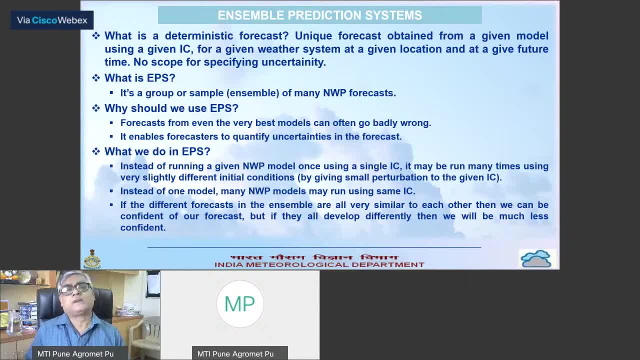 unique forecast obtained from a given unique forecast obtained from a given model. using a given ic model. using a given ic model, using a given ic, initial condition for a given weather. initial condition for a given weather. initial condition for a given weather system at a given location. system at a given location. 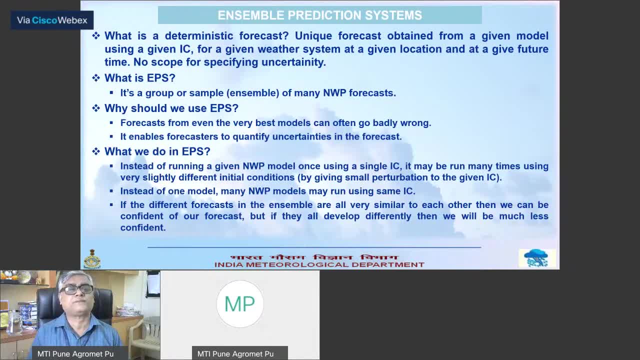 system at a given location and at a given future time: no scope for and at a given future time, no scope for and at a given future time, no scope for specifying uncertainty, specifying uncertainty, specifying uncertainty. eps: it is a group of eps, it is a group of eps, it is a group of group or a sample of many nwp forecast. 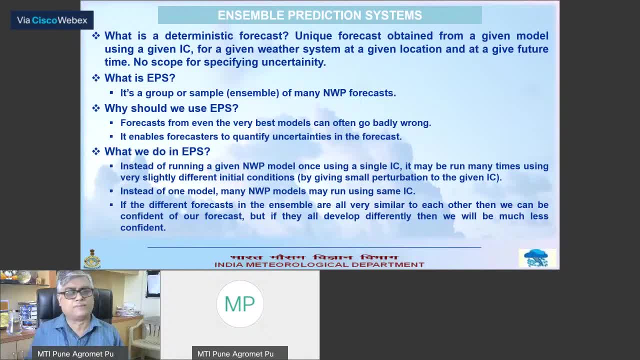 group, or a sample of many nwp forecast group, or a sample of many nwp forecast, but we don't use the word sampling you. but we don't use the word sampling you, but we don't use the word sampling. you know, we say ensemble, ensemble. why we should use ensemble? because 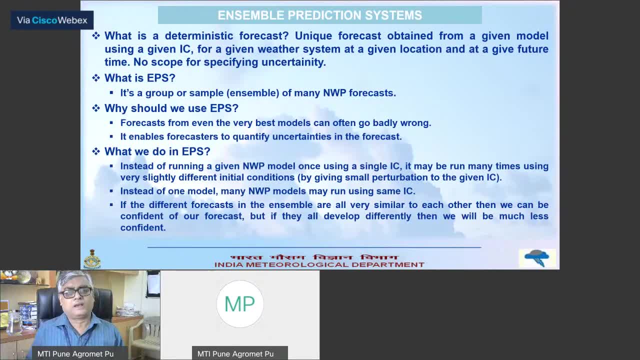 why we should use ensemble. because why we should use ensemble? because forecast as forecast, as forecast, as we have already discussed. we have, uh i'm. we have already discussed. we have, uh i'm. we have already discussed. we have, uh i'm seeing that forecast problem even very 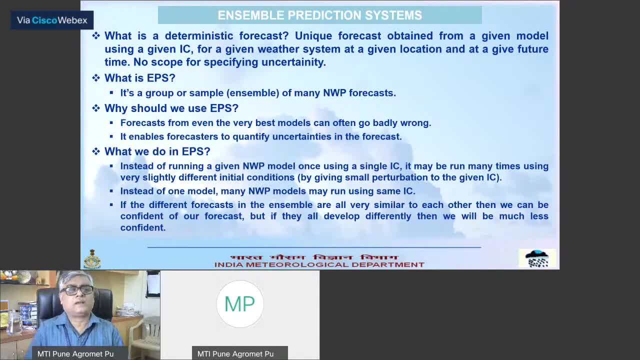 seeing that forecast problem, even very seeing that forecast problem, even very best model, best model, best model can go wrong and ensemble can go wrong and ensemble can go wrong and ensemble for prediction system enables the for prediction system, enables the for prediction system, enables the forecasters to quantify the. 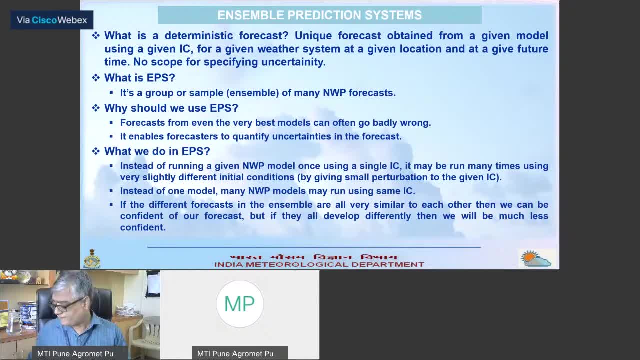 forecasters, to quantify the forecasters, to quantify the uncertainties in the future, what we do uncertainties in the future, what we do uncertainties in the future, what we do in the eps, in the eps, in the eps that i have, that i have, that i have. i have tried to explain. 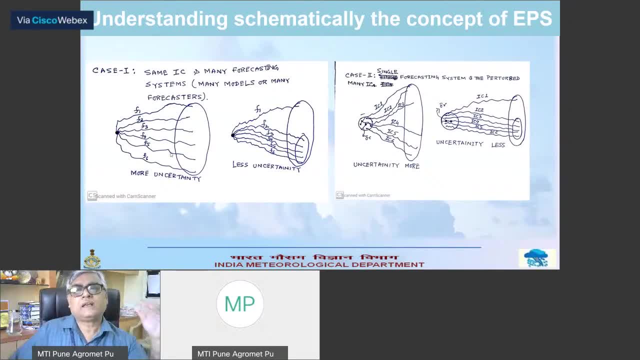 i have tried to explain. i have tried to explain in a schematic way, in a schematic way. in a schematic way: see to get a ensemble forecast. see to get a ensemble forecast. see to get a ensemble forecast for a given weather phenomenon at a, for a given weather phenomenon at a. 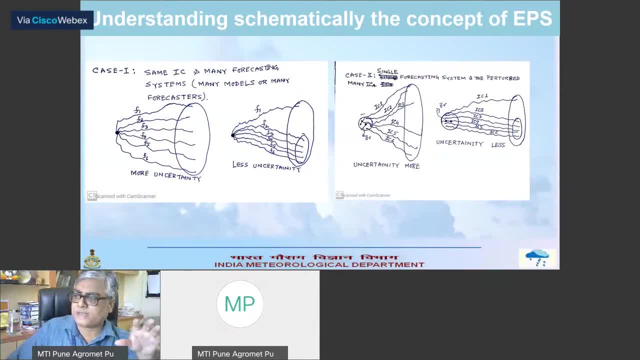 for a given weather phenomenon at a given place for a future, given place for a future. given place for a future, given future time. we should have a number given future time. we should have a number given future time. we should have a number of forecast, of forecast, of forecast. number of forecast for a for a given 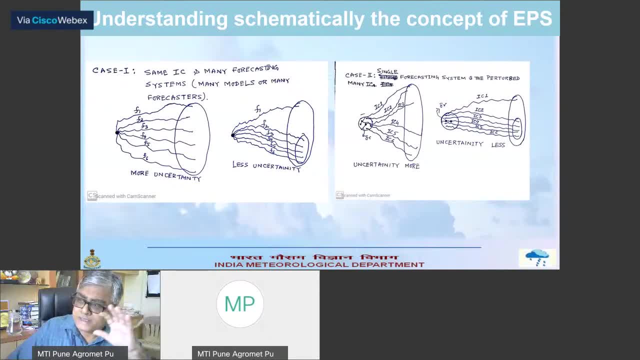 number of forecast for a for a given number of forecast for a for a given weather system at a given time. weather system at a given time, weather system at a given time. you, we can generate by two ways, one way. you, we can generate by two ways, one way. 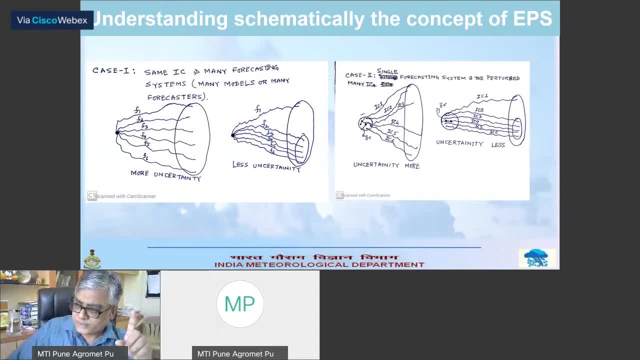 you. we can generate by two ways. one way is: is is one nwp model, one nwp model, one nwp model, but many initial but many initial but many initial condition condition condition. another one is same initial condition, another one is same initial condition, another one is same initial condition. many nwp models. 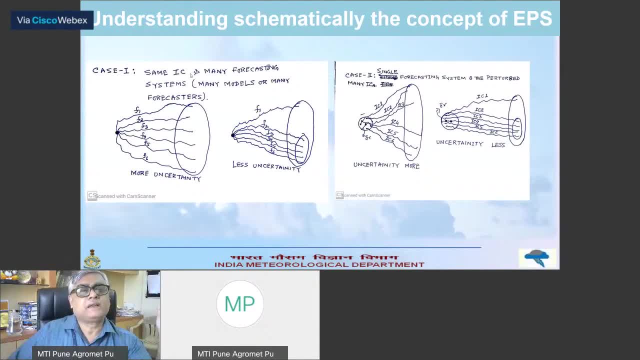 many nwp models, many nwp models. first case is initial condition is same. first case is initial condition is same. first case is initial condition is same and many forecasting systems we are and many forecasting systems we are and many forecasting systems we are having also imd forecasting system. 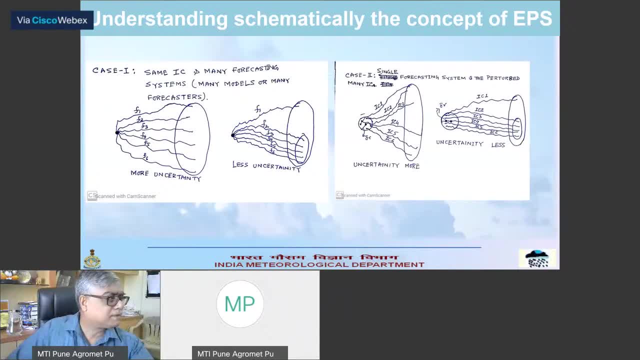 having also imd forecasting system. having also imd forecasting system, then nsf forecasting system, ecmwf, then nsf forecasting system, ecmwf, then nsf forecasting system, ecmwf, forecasting system, forecasting system, forecasting system. we see a double model. we say: model you. 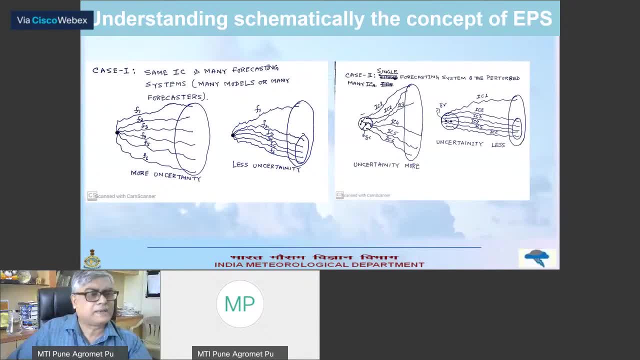 we see a double model, we say: model you. we see a double model, we say: model you came up with you, came at office model. came up with you, came at office model, came up with you, came at office model ecmwf model, etc. etc. so f1, f2, f3, f5, f6. 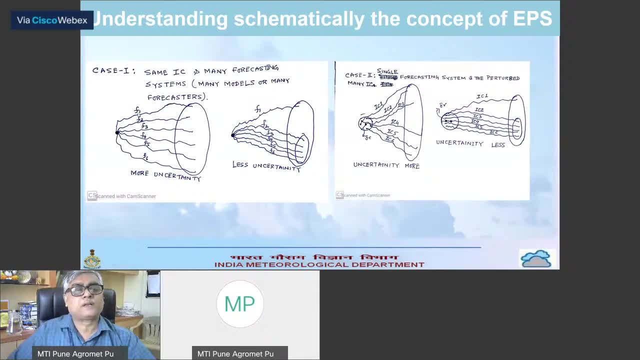 ecmwf model, etc, etc. so f1, f2, f3, f5, f6, ecmwf model, etc, etc. so f1, f2, f3, f5, f6, in both the picture they are all your in both the picture. they are all your in both the picture. they are all your different forecasting system, both all. 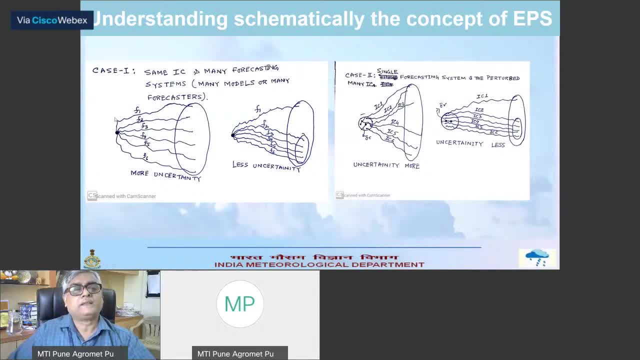 different forecasting system, both all different forecasting system, both all the forecasting system use the same the forecasting system, use the same the forecasting system, use the same initial condition and they are generating initial condition and they are generating initial condition and they are generating the forecast, the forecast, the forecast. these are the two cases. in this case, we 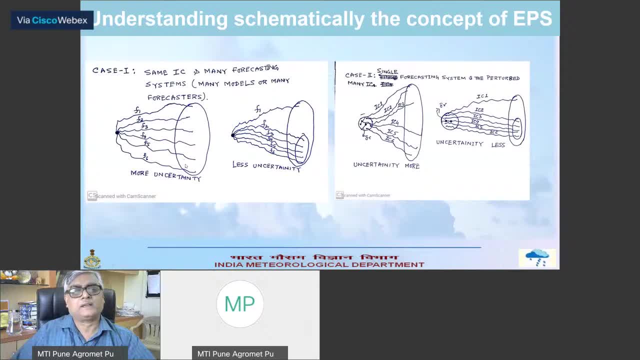 these are the two cases. in this case, we. these are the two cases. in this case, we can see all the forecast they are, can see all the forecast. they are, can see all the forecast. they are diverging from each other. here we see diverging from each other. here we see. 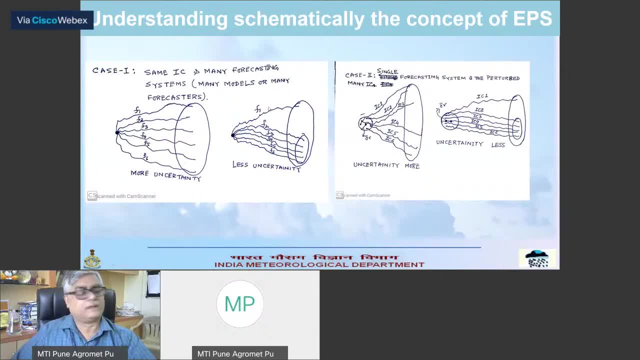 diverging from each other. here we see most of the forecast. are they are most of the forecast? are they are most of the forecast? are they are converging except one converging except one, converging except one. so quite natural, quite natural, uh. so quite natural, quite natural, uh. 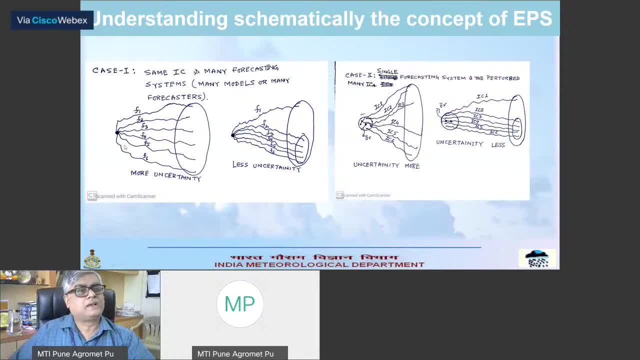 so quite natural, quite natural, uh, quite natural it has. quite natural, it has quite natural, it has less uh, less uh, less uh. it has more uncertainty, more uncertainty. it has more uncertainty, more uncertainty. it has more uncertainty, more uncertainty. and that means less reliable, and here it. and that means less reliable and here it. 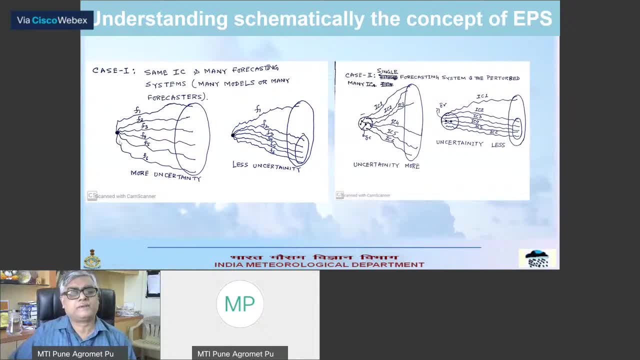 and that means less reliable. and here it is having, is having is having uh less uncertainty. here it was having uh less uncertainty, here it was having uh less uncertainty, here it was having more uncertainty, less uncertainty, so it is more uncertainty, less uncertainty, so it is more, more uncertainty, so it is more. 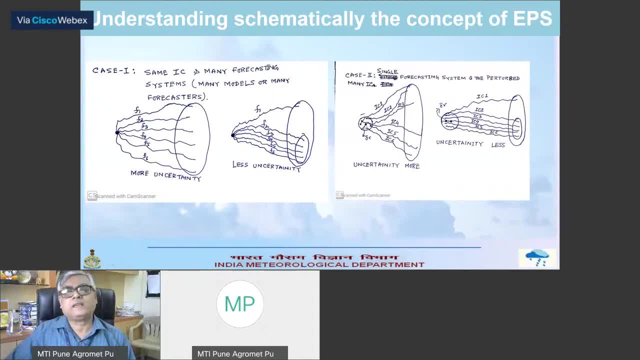 more uncertainty. so it is more relevant. case two is relevant. case two is relevant. case two is: i am having a single initial condition, i am having a single initial condition. i am having a single initial condition, single initial condition. these initial, single initial condition, these initial, single initial condition, these initial conditions are given. 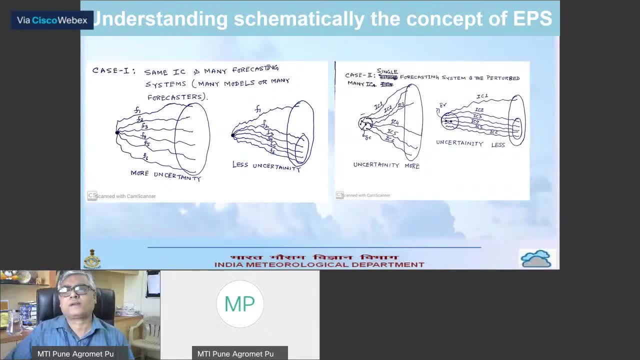 conditions are given. conditions are given infinite small perturbations, infinite small perturbations, infinite small perturbations. small perturbations are given. small perturbations are given. small perturbations are given. uh to the initial condition. it is very uh to the initial condition. it is very. 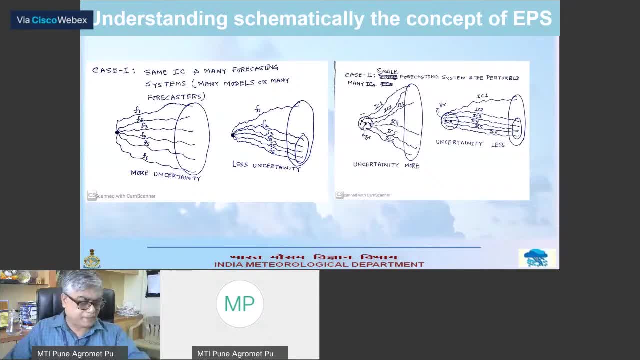 uh, to the initial condition. it is very simple thing, simple thing, simple thing: that whatever initial value of the that, whatever initial value of the that, whatever initial value of the metallurgical parameter, we have already metallurgical parameter. we have already metallurgical parameter, we have already having. 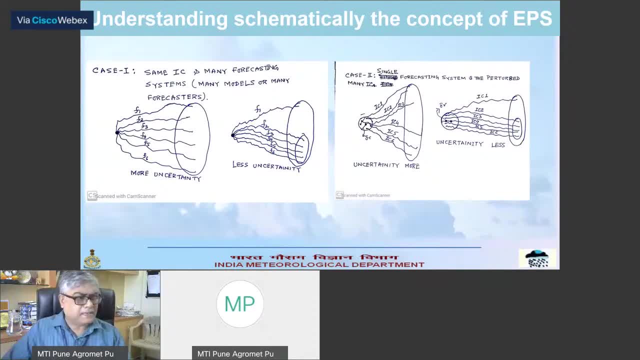 having having from that, by changing a little bit from that, by changing a little bit from that, by changing a little bit, let me, let us let, let us generate many. let me, let us, let, let us generate many. let me, let us let let us generate many values of those metallurgical parameters. 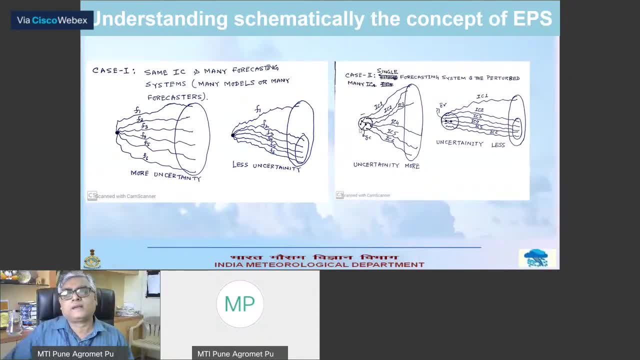 values of those metallurgical parameters. values of those metallurgical parameters, so, but we have to remember that, uh, this so, but we have to remember that, uh, this so, but we have to remember that, uh, this magnitude of the perturbation should be, magnitude of the perturbation should be. 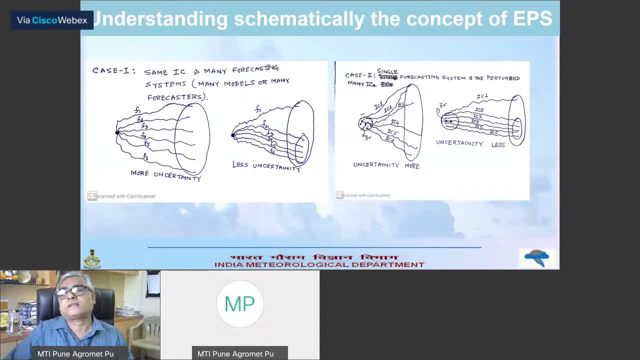 magnitude of the perturbation should be small. so, therefore, that's why i have small, so, therefore, that's why i have small. so, therefore, that's why i have what i have done here, centered at the, what i have done here, centered at the what i have done here, centered at the initial condition. 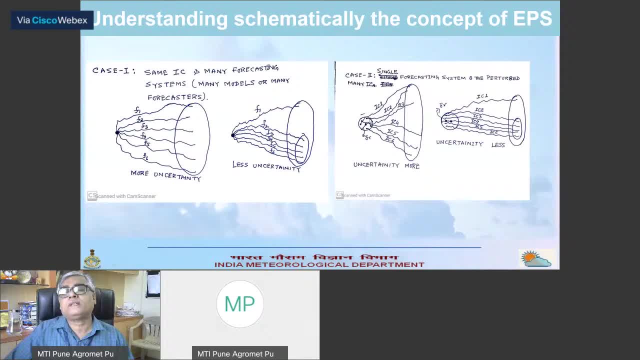 initial condition, initial condition: i have drawn a circle with infinitesimal. i have drawn a circle with infinitesimal. i have drawn a circle with infinitesimal radius and within that radio, within that radius and within that radio, within that radius and within that radio, within that circle, only all perturbations. 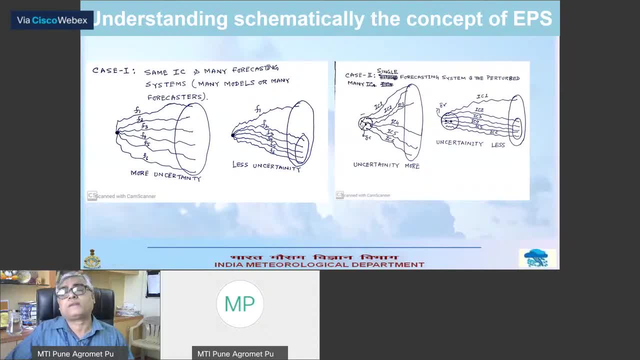 circle, only all perturbations circle, only all perturbations perturbed. initial conditions should be perturbed. initial conditions should be perturbed. initial conditions should be there and using all the perturbed initial there and using all the perturbed initial there and using all the perturbed initial condition. 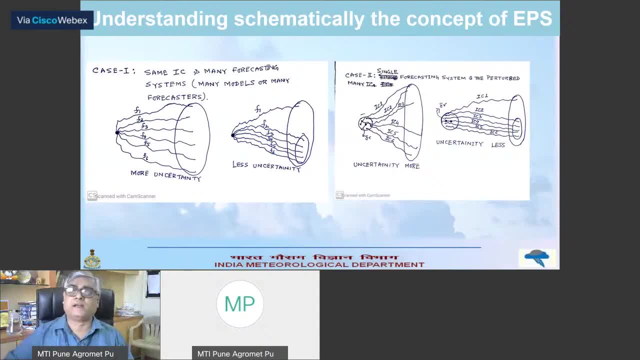 condition condition in initial condition in initial condition in initial condition, same model is being run. so that is any same model is being run. so that is any same model is being run. so that is any model run with initial condition: one, two model run with initial condition: one, two. 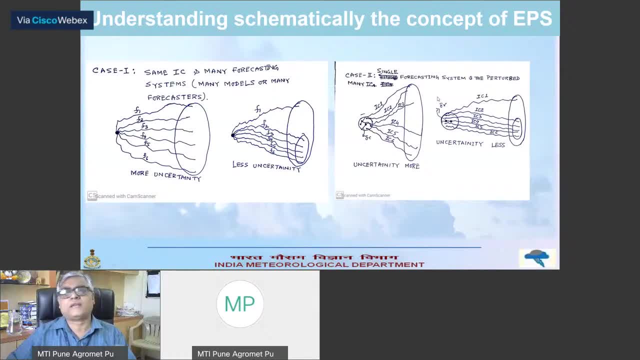 model run with initial condition: one, two, three, etc, etc. we can. we can have the three, etc, etc. we can. we can have the three, etc, etc, etc. we can. we can have the different types of situation, two different types of situation, two different types of situation, two situation. i have shown, in any case, we 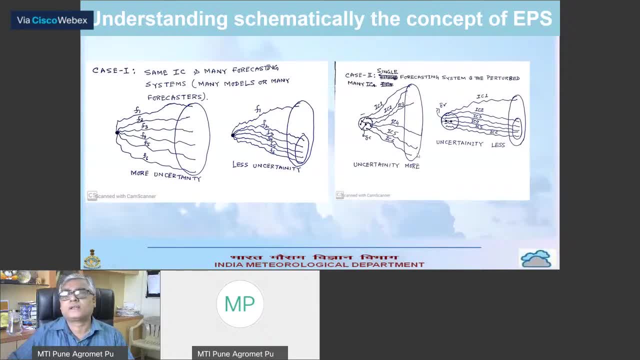 situation i have shown, in any case, we situation i have shown, in any case, we can, can, can very easily see in these situations, very easily see in these situations, very easily see in these situations forecasts are diverging from each other, forecasts are diverging from each other. 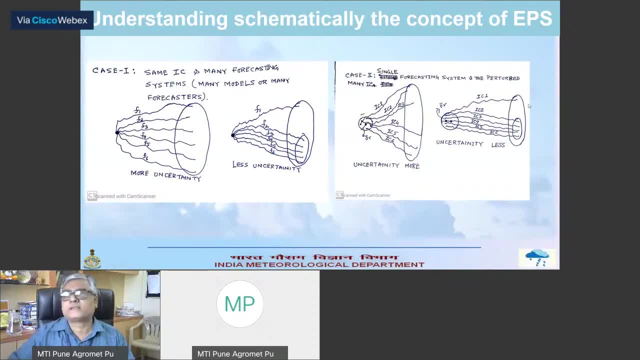 forecasts are diverging from each other: having more uncertainty and here it is having more uncertainty, and here it is having more uncertainty and here it is less uncertain. it's just that definitely less uncertain. it's just that definitely less uncertain. it's just that definitely. giving a single, even not only that, using 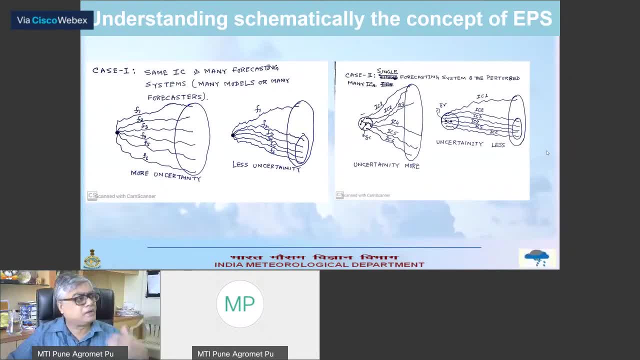 giving a single even. not only that. using giving a single even. not only that, using many forecast, we can do lot of probability, many forecast. we can do lot of probability, many forecast. we can do lot of probability um a lot of statistics also. we um a lot of statistics also we. 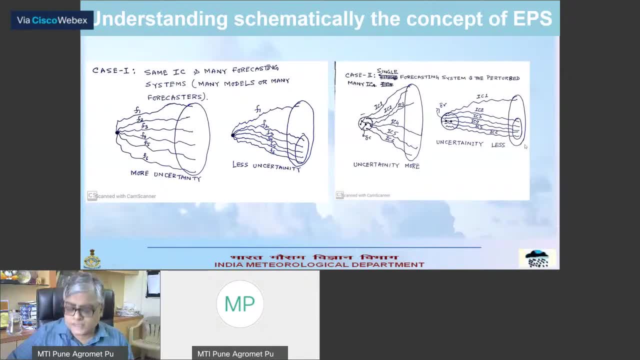 um a lot of statistics also, we can find out the what is the focus mean, can find out the what is the focus mean, can find out the what is the focus mean. what is the focus? what is the focus mean? what is the focus mean? ensemble mean. what is the ensemble spread? 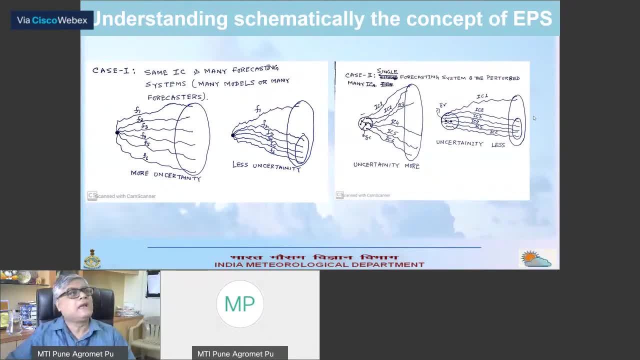 ensemble mean: what is the ensemble spread? ensemble mean: what is the ensemble spread? that is standard variation. that is standard variation. that is standard variation. variance, how much it is there, and variance, how much it is there, and variance, how much it is there. and different probability distribution also. 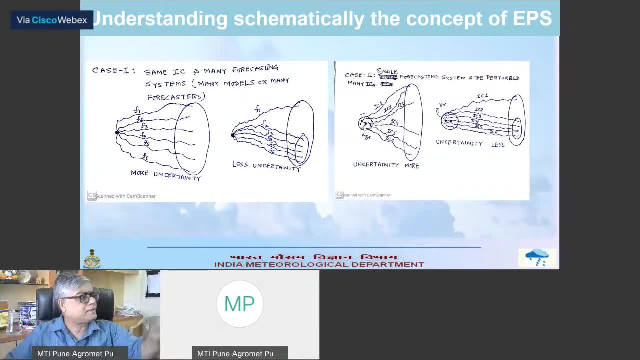 different probability distribution also. different probability distribution also. what is the probability of 75 percent? what is the probability of 75 percent? what is the probability of 75 percent uh? what is the probability of uh? what is the probability of uh? what is the probability of a heavy rainfall? what is the probability of? 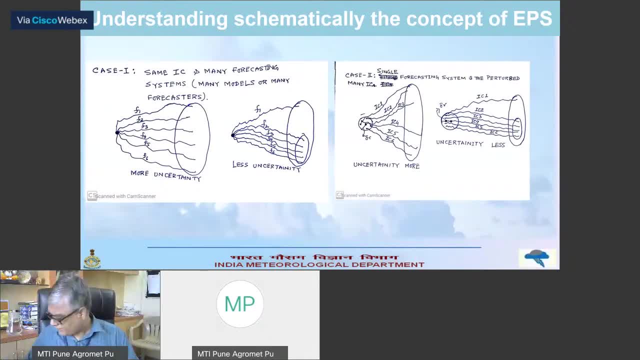 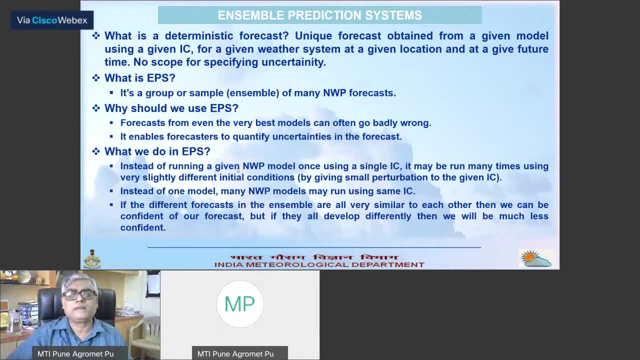 less rainfall, like that, like that, so that only what we do in the eps, that is same thing, only it is written. instead of running a given nwp model once once using a single initial condition, it may be run many times using very slightly different initial condition. otherwise, instead of one model run, many model nwp models may run using same initial condition. 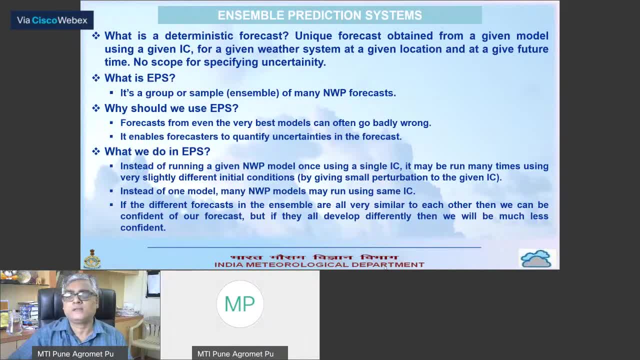 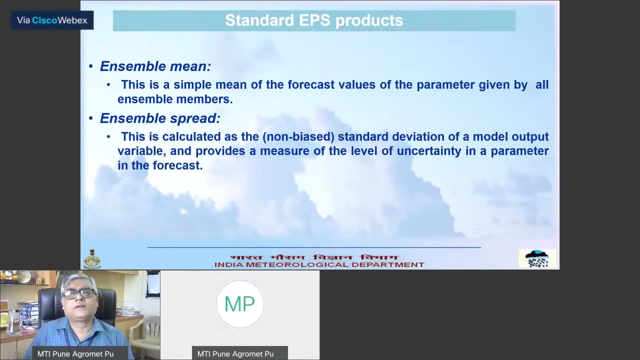 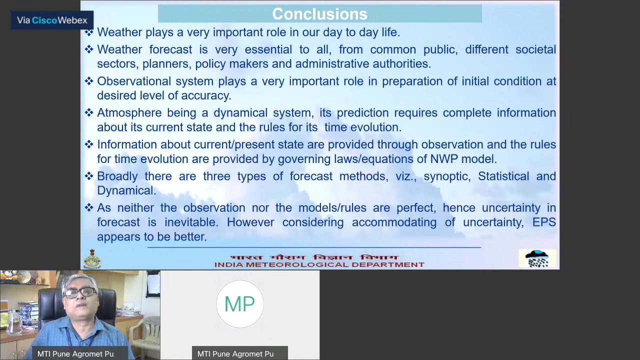 if the different focus in the ensemble are all very similar to each other, then we can be confident of our focus. if they all develop differently with time, then we will have less confident. and these are the different. product is, as i told, ensemble mean ensemble spread, etc. and i am now at the flag end of the my presentation conclusions. 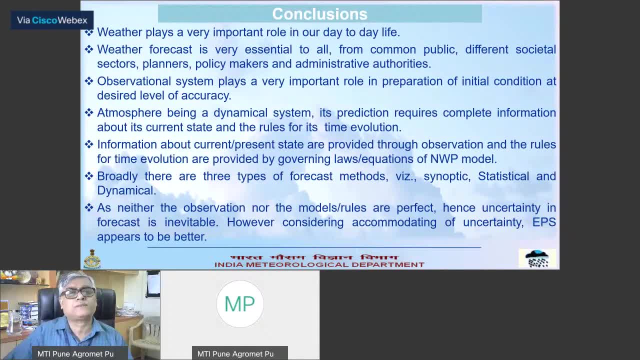 from our discussions what we have found, that, whether of code, it plays a very important role in our day-to-day life, forecast weather is very much essential to all sectors- societal sectors- and observational system plays a very important role in preparation of the initial condition at desired level of accuracy and atmosphere, being a dynamical system. 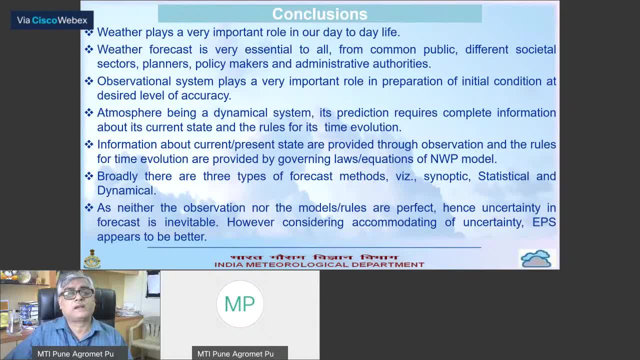 it. prediction requires complete information about the current state and the rules for its time evolution, which are provided by governing equations and the initial conditions. information about current state i have already told. i have broadly. there are three types of focus: synoptic, statistical and dynamical. as neither the observation not the model rules are, 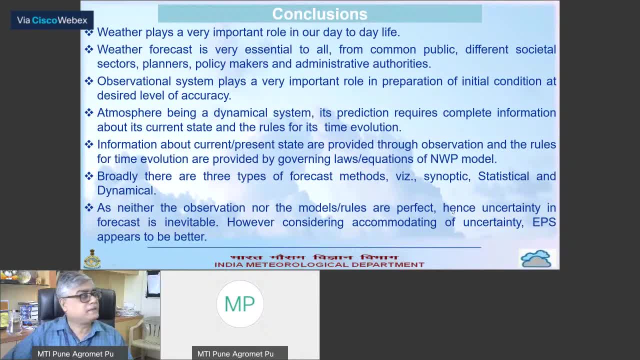 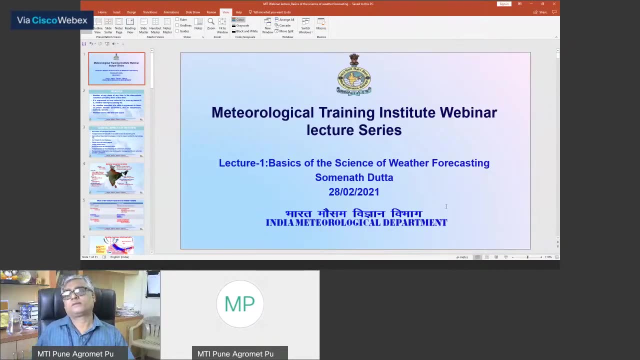 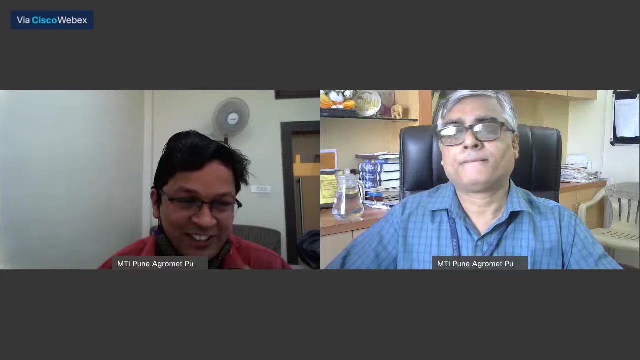 perfect models or rules are perfect, so uncertainty is inevitable. however, considering the accommodating of uncertainty, eps appears to be better. thank you, thank you, series. i have finished. thank you, sir. thank you very much for your valuable guidance and it is for how that the entire, or we, can now think that you should get more knowledge from your lecture. So, sir, we got.